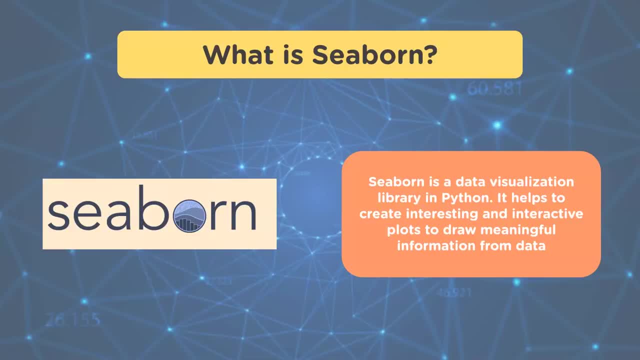 and how to create different plots and know the data better. we'll look at the Seaborn library in Python. We'll be using two datasets in our demo. The first one is the empty-cast dataset and the second is the popular iris flower dataset. Now let's head over to our 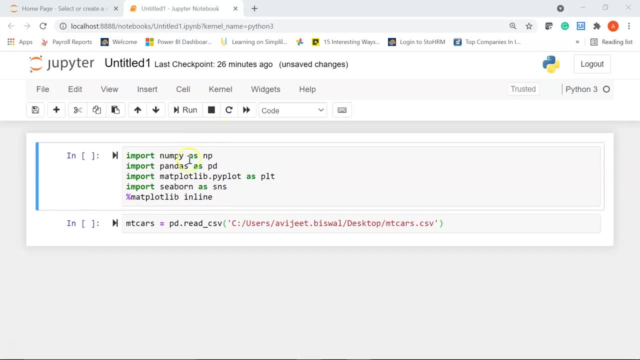 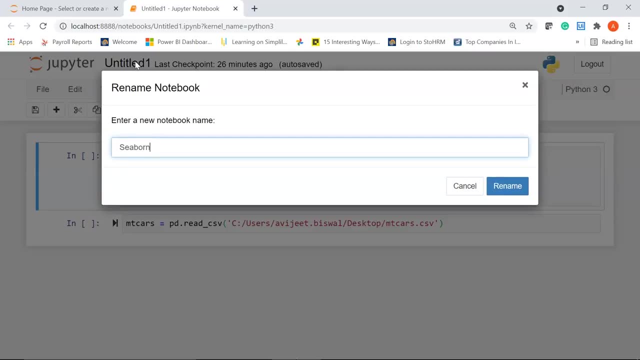 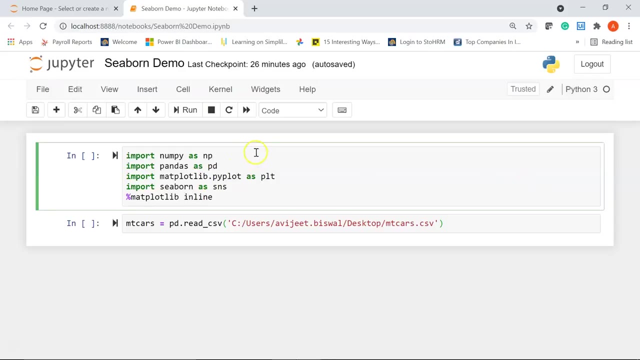 Jupyter notebook and start with our demonstration. So I am on my Jupyter notebook. Let me go ahead and rename the notebook. I'll say Seaborn demo. We'll rename it. Alright, You can see it's already filled in. So while working on an exploratory data analysis project using 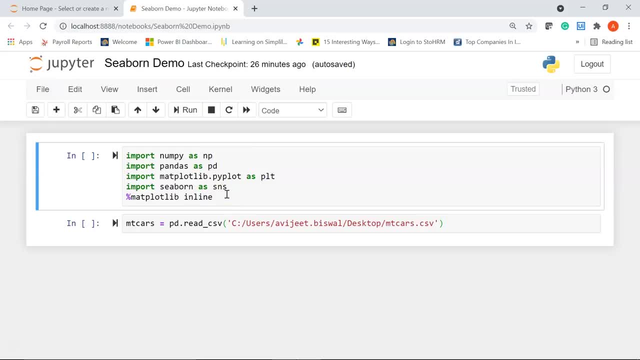 Python. you will need NumPy, Pandas, Matplotlib and Seaborn libraries for data manipulation and visualization. So let's import these libraries first. So I've already written: import NumPy as np, Pandas as pd, Matplotlibpyplot as plt, Seaborn as sns. Alright, So I'll hit. 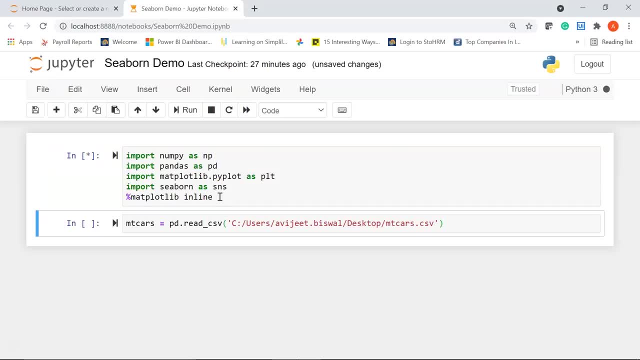 shift enter to run this first cell. Alright, Now, using the read underscore csv function that is present in the Pandas library, I am importing my dataset that is empty-cast. I'll tell you what empty-cast is about. This is a csv dataset, and here I have given the location where my dataset is present. Let's run it. 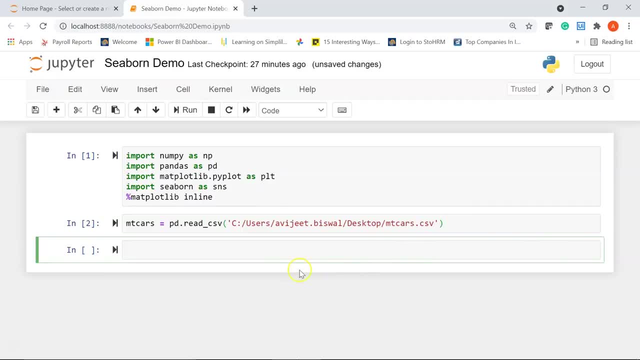 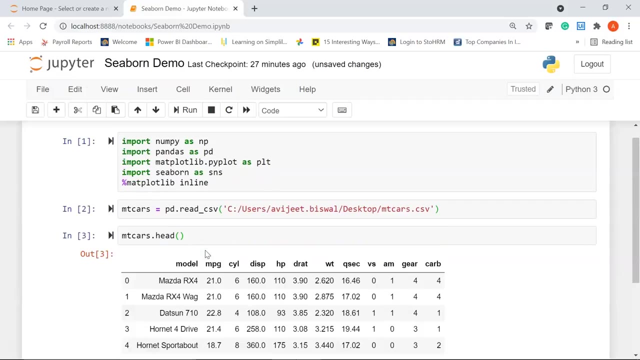 Alright, Now let me go ahead and print the first five rows of my empty-cast dataset. Alright, So I've taken the data frame. For that I am using the head function. If I run it, Okay, You can see here, it has given me the first five rows. The index starts from zero till. 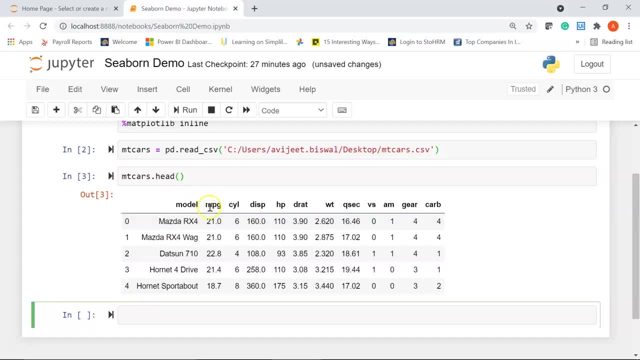 four, So total five rows of information, And you can see these are the columns that are present in the empty-cast dataset. The first is the model of the car. Now just let me give you a background about this dataset. So the data is taken from the 1970s. 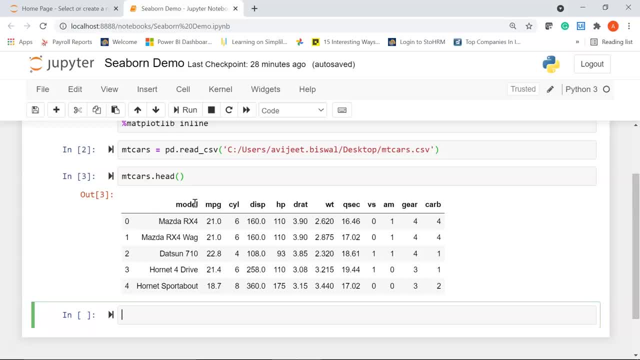 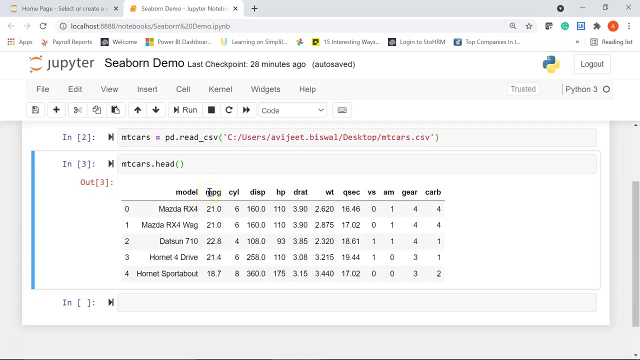 It is in 1974, motor trend US magazine. It has information about fuel consumption and eleven different aspects of automobile design and performance of 32 cars, Alright. So here we have the first column as the model of the car, and then we have MPG. 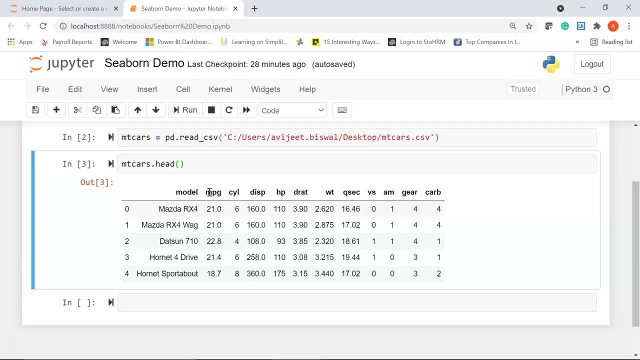 which is miles per gallon. Then we have CYL, which stands for the number of cylinders in the vehicle or the car. Then we have DISP, which is displacement, up to an inch. Then we in cubic inches. so these all values are in cubic inches. after that we have HP. 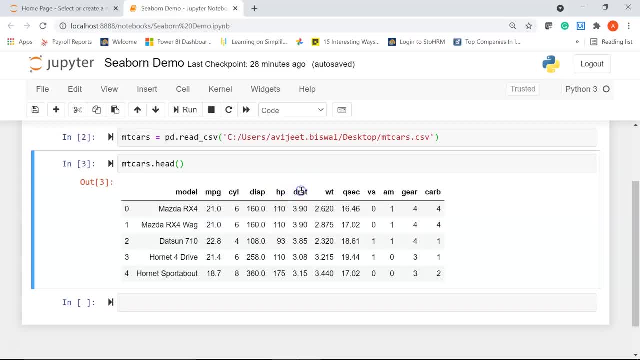 which is gross horsepower. then we have something called as dr80, which is basically the rear axle ratio. then we have WT, which is the weight of the car in pounds, so think of it as weight multiplied by thousand pounds, all right. and then we have QSEC, which is one-fourth mile time. this is a measure. 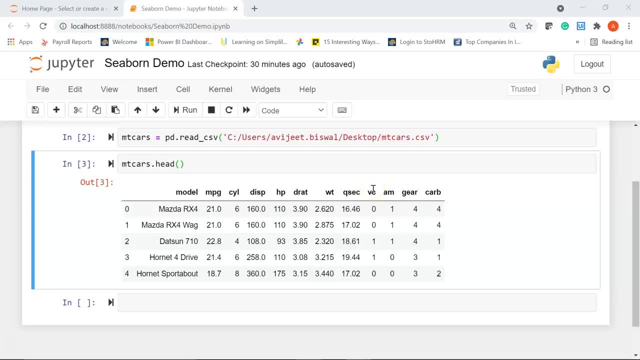 for acceleration. then we have something called as VS. this is the type of engine for each of the vehicles, so zero stands for V shaped engine and one stands for straight engine. then we have AM, which is basically the mode of transmission. so zero is for automatic transmission and 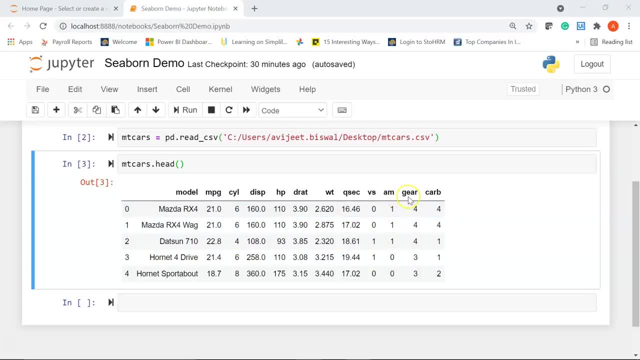 one is for manual transmission. then we have the number of forward gears present in the vehicle, and then we have something called as CARB or C A R B. this stands for the number of carburetors. so carburetors is a device for supplying a spark ignition engine with a mixture of fuel and air. all right, 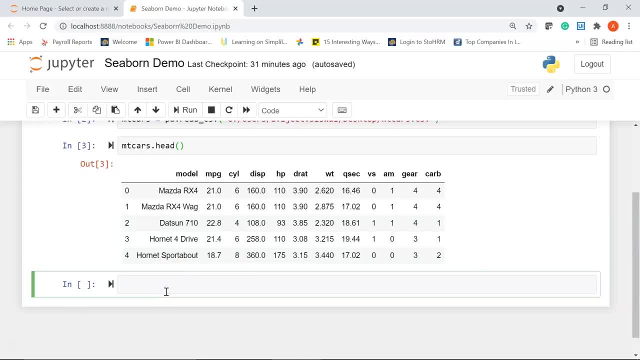 now let's talk about the fuel and the air. then we will jump to the environmental data type. now we will use the info function to print the summary of the data frame. so the info function returns information regarding the index data type column data types. then we have the 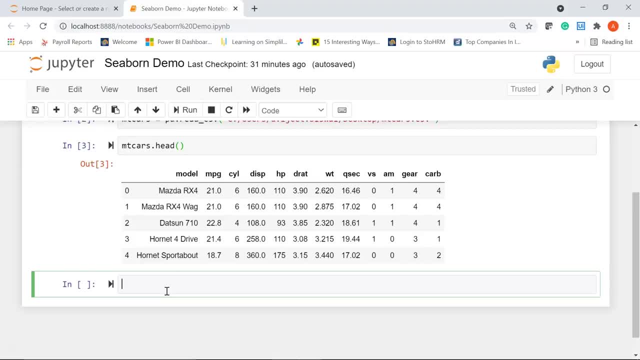 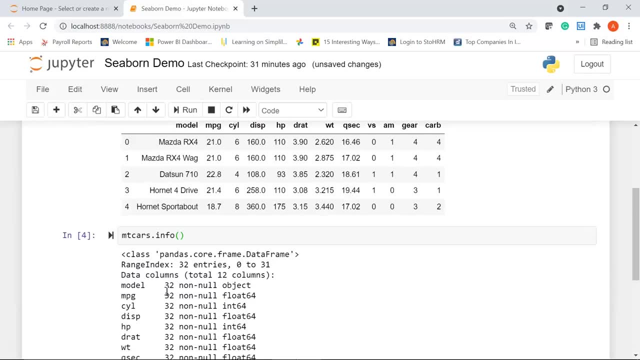 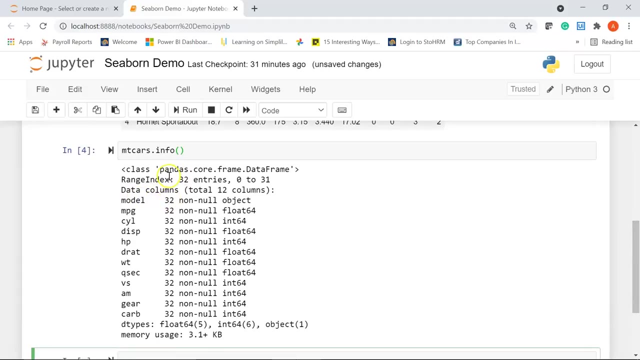 information about non non values and memory usage. so I'll write my data frame name, which is empty-cars dot. I am going to use the info function. let's run it and here you can see. we have all the columns. there are total 32 and H, two different values. if you have the rightанные values. 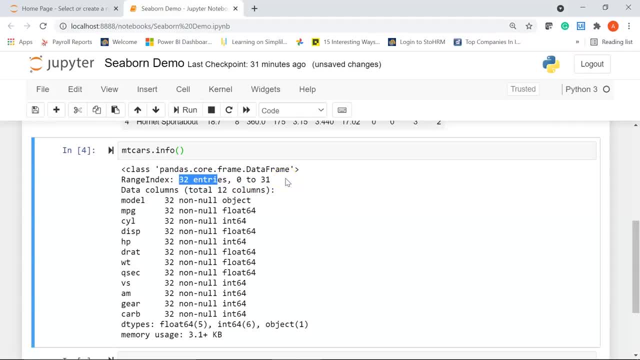 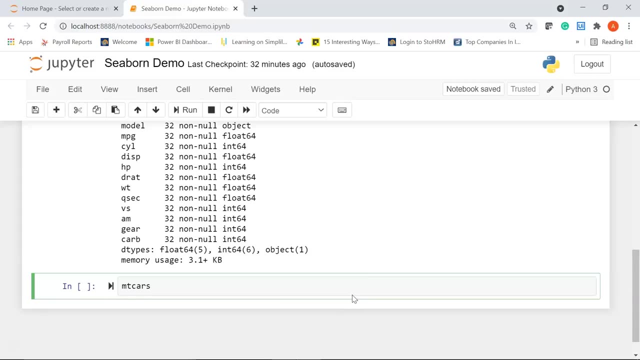 entries from 0 to 31, so data about 32 cars. then here you can see the data types and the memory usage. now, moving ahead, let me just print the shape of the data frame. that will give you the number of rows and columns present. I'll use the 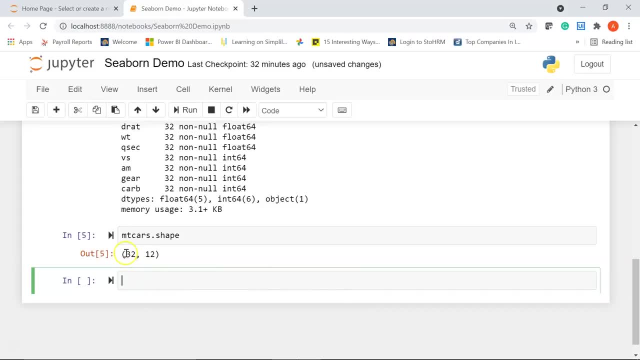 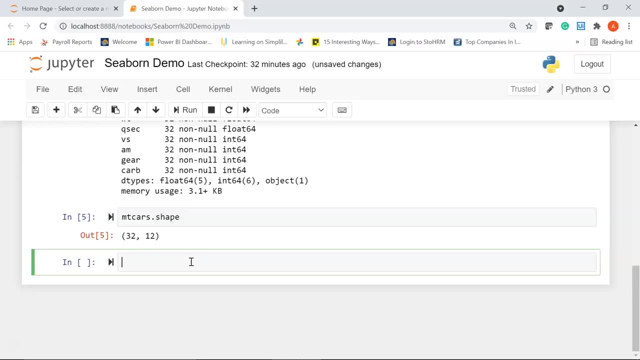 shape attribute. you can see here there are total 32 rows and 12 columns in my data set. now the seaborn library provides a range of plotting functions that makes the visualization and analysis of data easier. so we will cover some of the crucial plots that are available in seaborn. so let's start with. 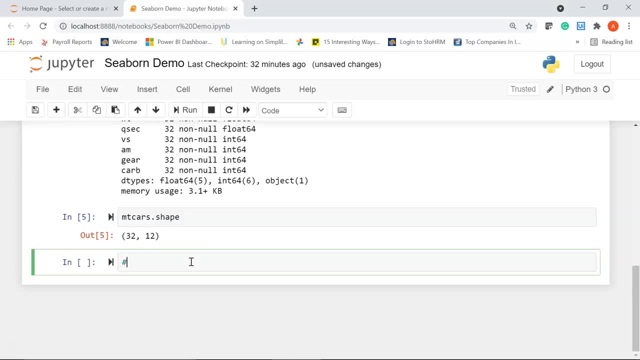 a bar plot. I'll give a comment as bar plot now. first understand what a bar plot is. so a bar plot gives an estimate of the central tendency of a numeric variable with the height of each rectangle. it provides some indication of the uncertainty around the estimate, using error bars. now to build this plot, you. 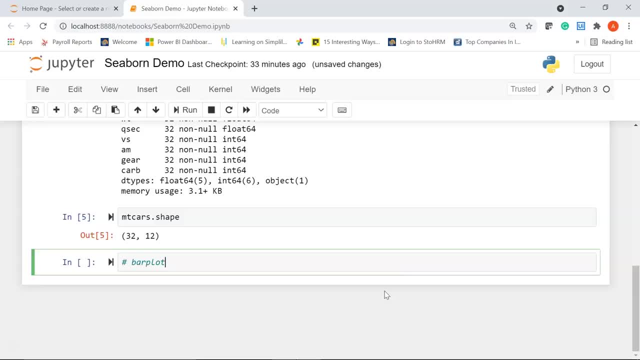 usually choose a categorical column in the x-axis and a numeric column on the y axis. so we'll create a bar plot between the number of cylinders and the miles per gallon. so let's start. I'll declare a variable called res, which essentially stands for result. then I'll use SNS, which is for the seaborn library. I'll say: 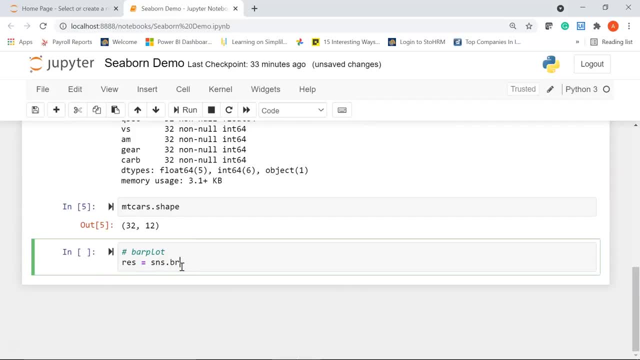 SNS dot, followed by my bar plot function, and inside the function I'll pass in my data frame name, that is empty cars, and then for x-axis, within the bracket you can see that my data frame name is empty cars, and then for y-axis I'll say my data. 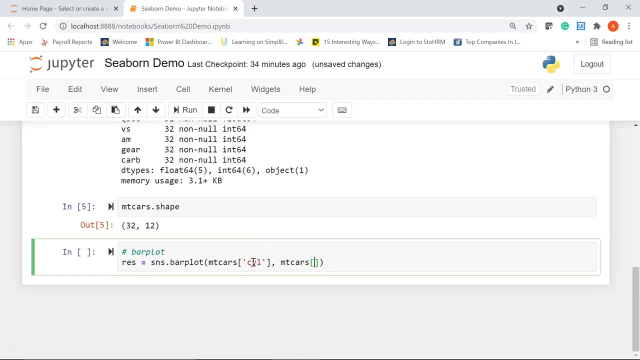 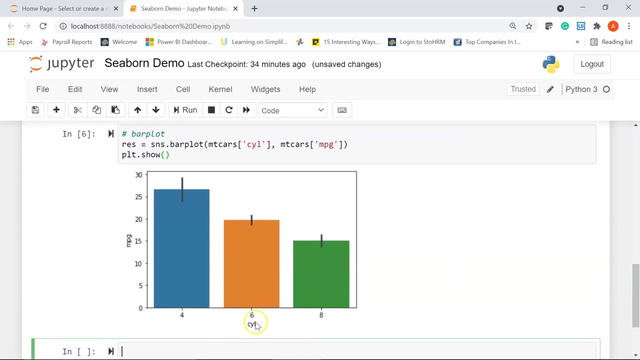 frame name empty cars, then the square bracket, followed by my y-axis column, that is miles per gallon. now to display, I'm going to use the matplotlib function. I'll say PLT dot show. let's run it and we'll see the result. there you go, so here you can see. on the x-axis we have the number of cylinders. 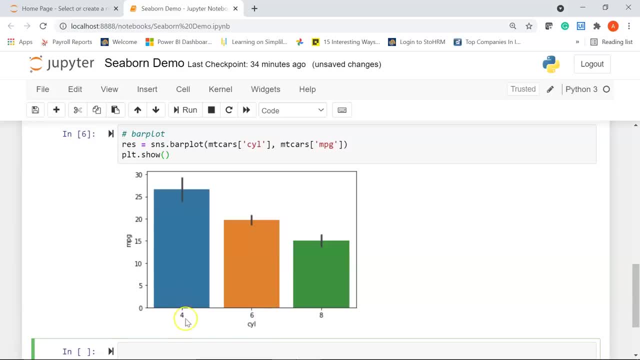 so in our data we have vehicles with four, six or eight cylinders, and on the y axis you can see the miles per gallon. now what essentially this graph tells us is that when the number of cylinders in the vehicle increases, my miles per gallon on mpg for the vehicles decreases, and you can see these. 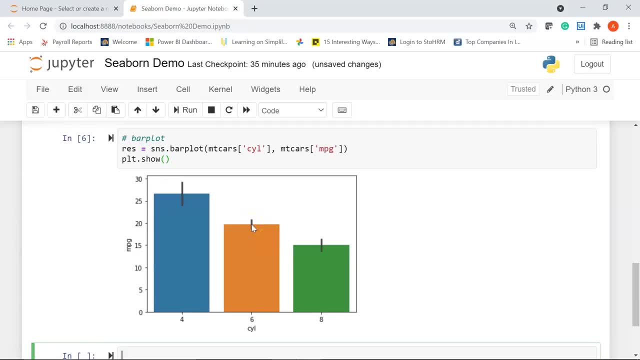 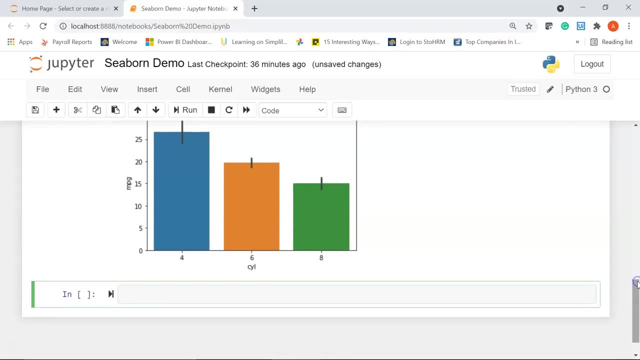 black lines. so these lines indicate the uncertainty around the estimate using error bars. all right, now you can create the same bar plot using another way. now we will exclusively define the x and y axis columns and also pass the name of the data frame using the data argument. let me show you how to do it. I'll use: 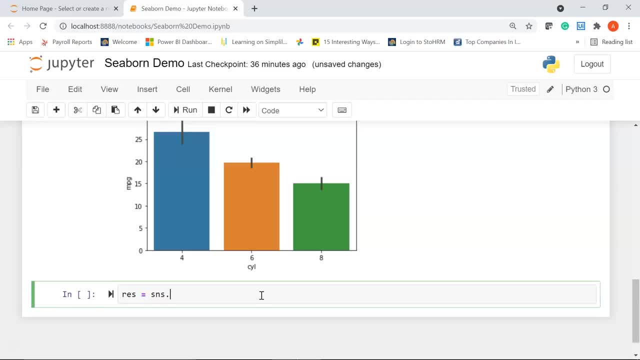 the same variable name are: yes, which stands for the data frame, and the data stands for result. I'll say SNS dot bar plot. now, inside the bar plot function, I'm going to exclusively define my x-axis. I'll say x equal to, I'll pass in. 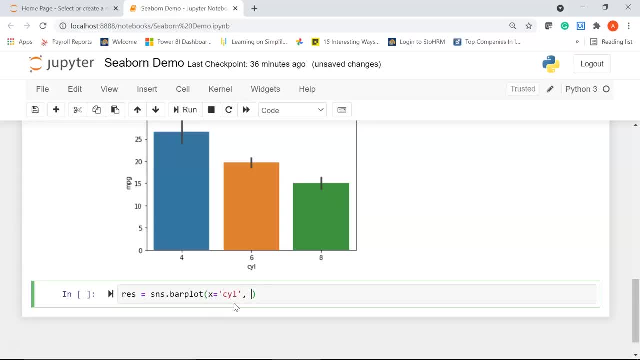 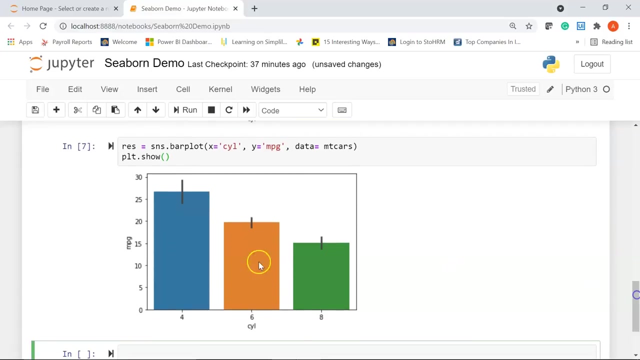 my column as cylinder, then I'll say y axis, which is miles per gallon, and then, using the data attribute, I'll pass in my data frame name that is empty cars, and finally we'll write PLT dot show. let me run it. you see, here we have the exact same bar plot as the above one. so this is another way to. 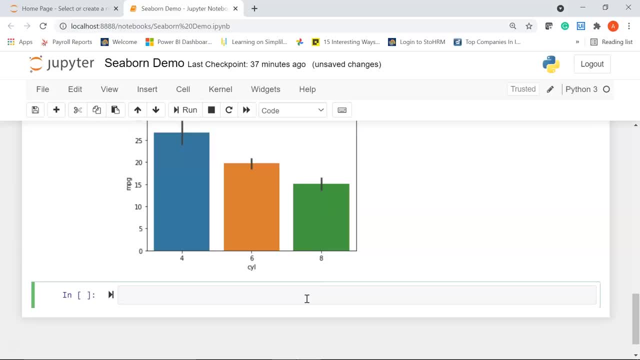 create a bar plot. now, Python seaborn allows the users to assign colors to the bars. so the bar chart that we are going to create will convert all the bars to a particular color. so for that I am going to use the color argument and then I'll use the color argument. so I'll say R ES equal to SNS dot. my function, that is bar. 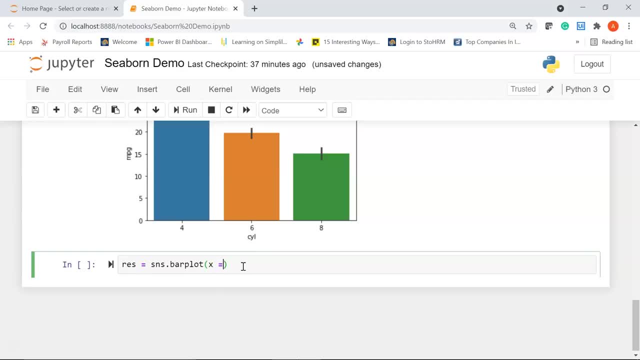 plot. I'll say X equal to cylinder, my y-axis will have mpg. then I'll say: data is empty, cars give a comma. and my final attribute: I'll say color equal to. I'll say yellow, close the bracket. and then I'm going to write PLT dot show. if I run it, you can. 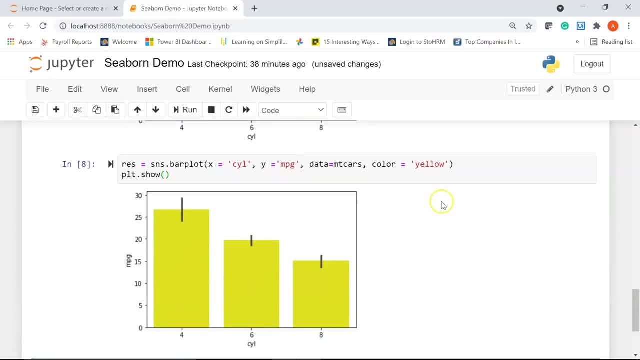 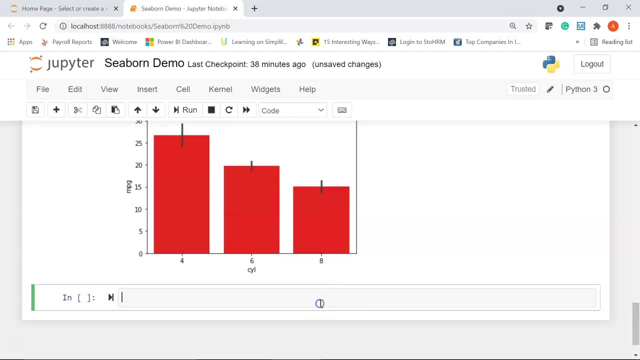 see here: all the bars have been converted to yellow color. now you can change the color argument. let's say, I'll make it to red if I print it. you can see here: all the bars have been changed to red color now. all right, now seaborn library also has the palette argument which you can use. 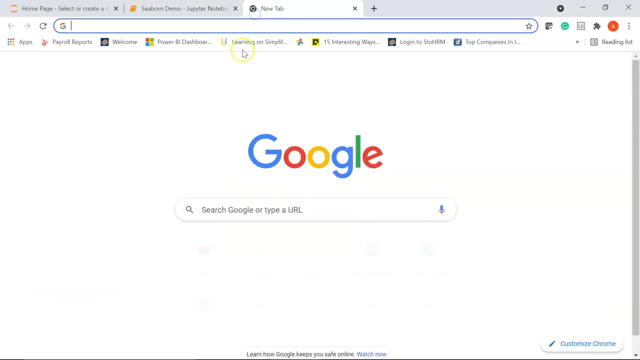 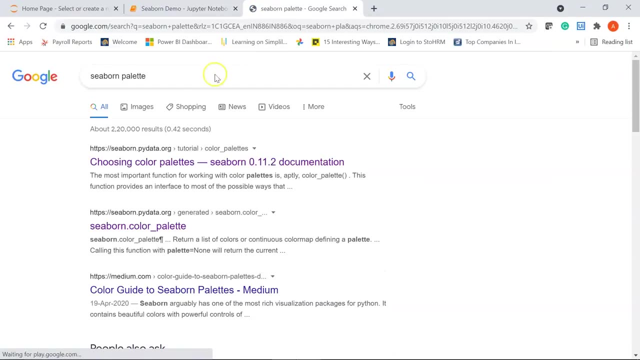 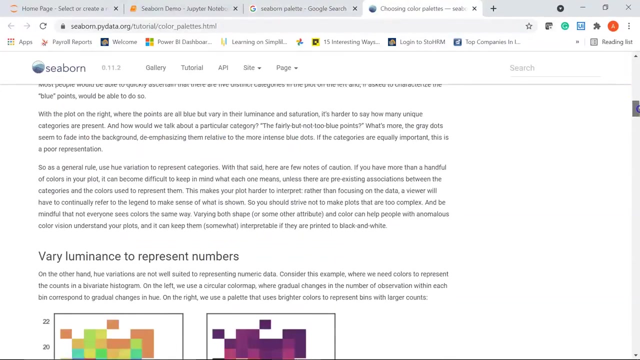 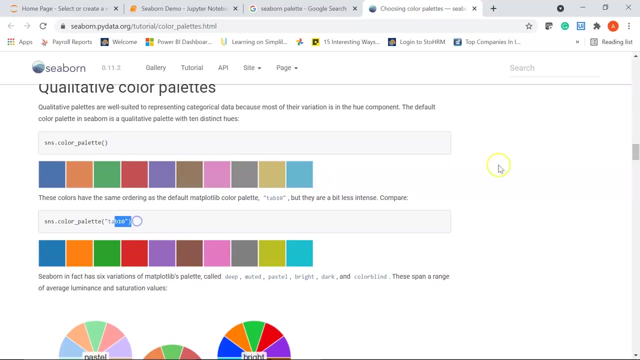 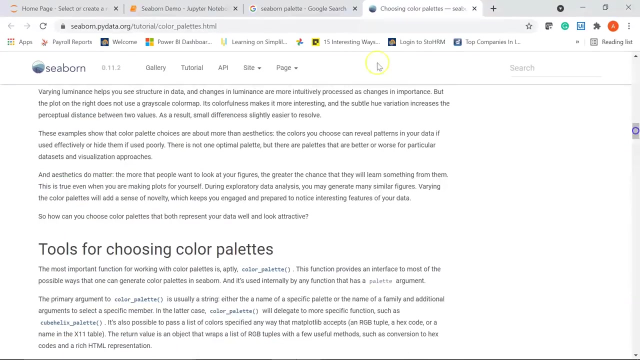 to give different colors to the bars. so if you go to Google and search for seaborn palette, you have a nice link here. so here you have. there are different palettes provided by seaborn. you can see here SNS dot color palette and these are the names of the palette. you can use whichever palette you want, all right. so 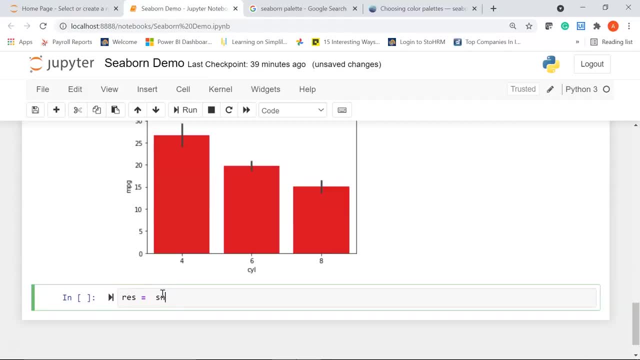 I'll say R ES equal to SNS dot bar plot. we'll use our first method of assigning a bar plot. so I'm using my data frame- empty cars- and this time we are going to change the X and Y labels. let's say I'm using my X label as: 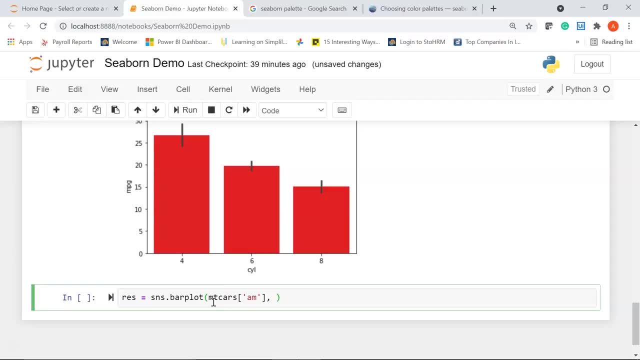 transmission, whether automatic or manual transmission, and then in my y-axis I'll have miles per gallon. then I'm going to say palette equal to- let me do spelling mistake here. let's say: our palette is set to. this is the name of the palette. I'll write PLT dot show. if I run it, you. 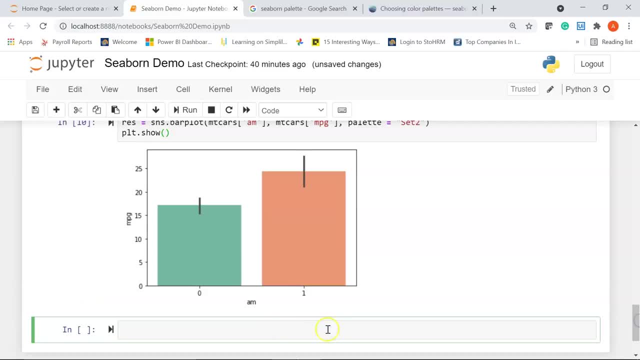 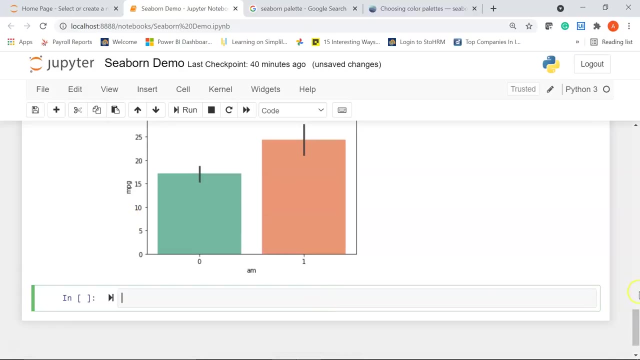 can see. here we have the two modes of transmission. zero is for automatic transmission of the vehicle, one is for manual transmission and the other is for manual transmission and you can see the miles per gallon for each of the modes of transmission. if you want, you can change the palette colors. let me just 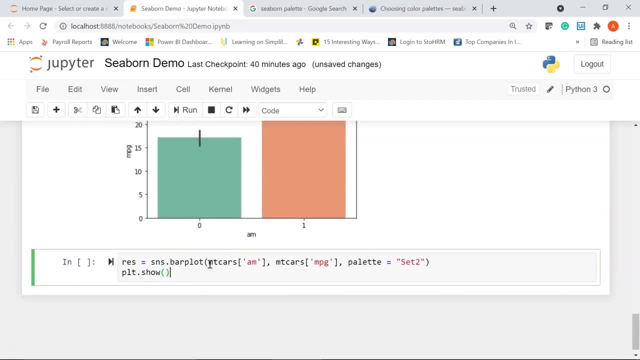 copy this, I'll paste it in my new cell and instead of set to, let's say, we'll use another palette called as a rocket, and I'm also going to alter my X and Y labels. let's say, in my X label I'll have gear and my Y label will be horse. 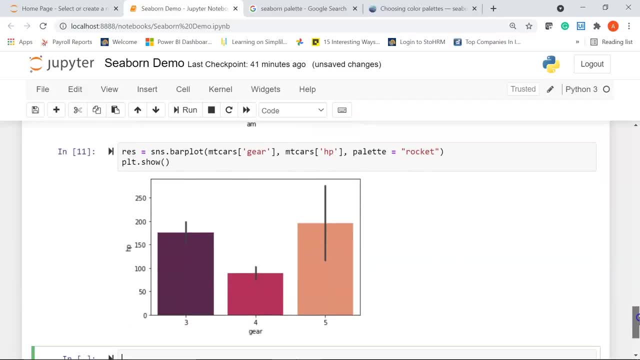 bar. if I run it. you see here we now have a different palette and the bars are of different colors. on the x-axis you have the gears 3 gear, 4 gear or 5 gear, vehicle, and on the y-axis you have the horse bar. so from the graph you can see. 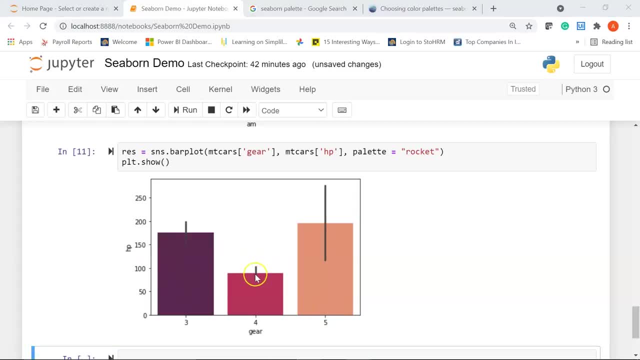 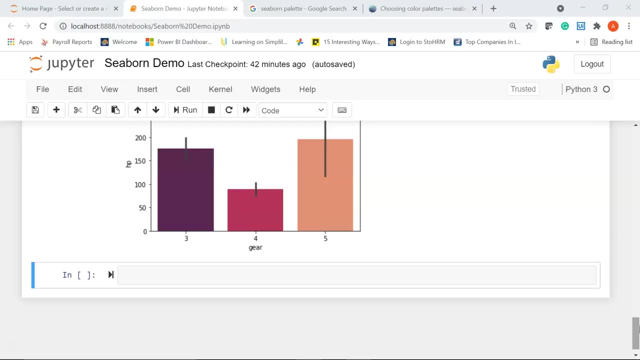 the horse bar is low for vehicles that have 4 gears, while it is high for the vehicles that have 5 gears. now let's understand how to create a count plot. so the count plot function in the Python seaborn library returns the count of total values for each category using bars. we will create a count plot that. 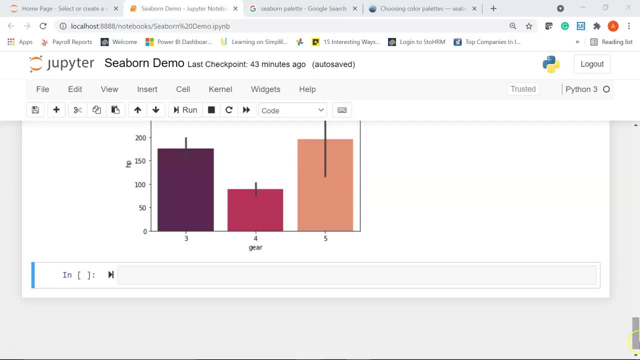 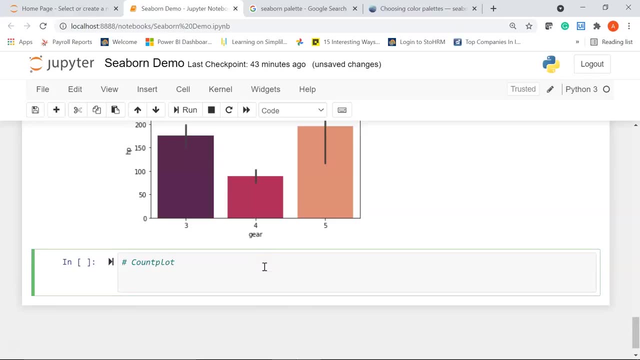 returns the total number of vehicles for each category of cylinders. I'll just give a comment here at faithful and at course I'll also give a comment for its count plot. all right, so I'll start SNS dot, I'll use the count plot function and I'll define my. 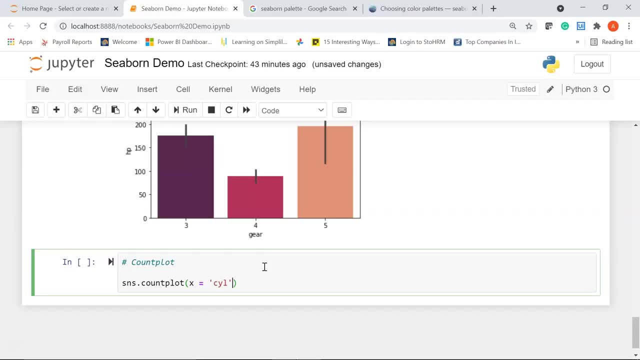 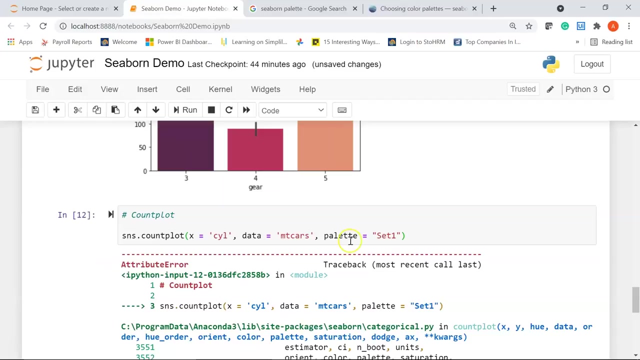 X axis as cylinders. my y-axis won't have any label or any column because y-axis will only show the count. then I'm going to use my data parameter or the argument and pass in my data frame name that is empty cars. let's say I will set the palette to set one. let me run it okay. 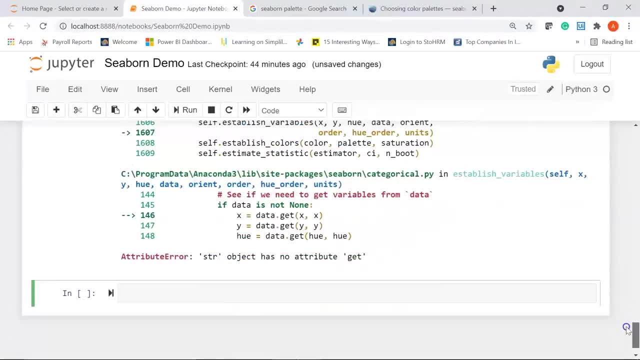 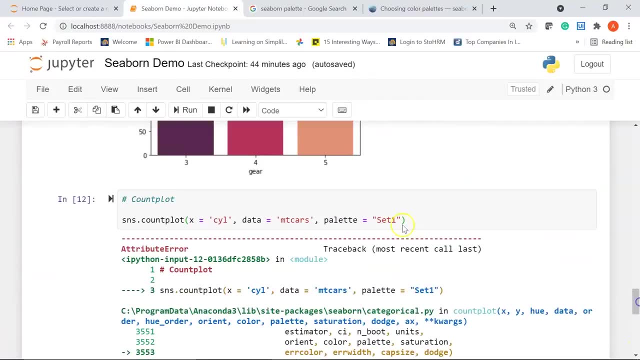 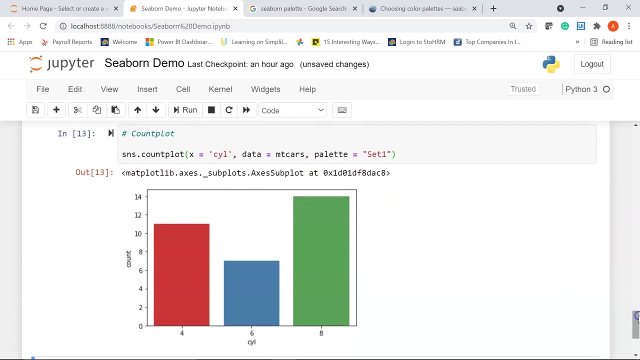 there is some error. let's debug the error. it says str object has no attribute get. okay, so this should be without the single quotes. make sure the data frame name is without the single quotes. let's run it again. there you go, so you can see here. this is a nice count plot that shows the number of cylinders on. 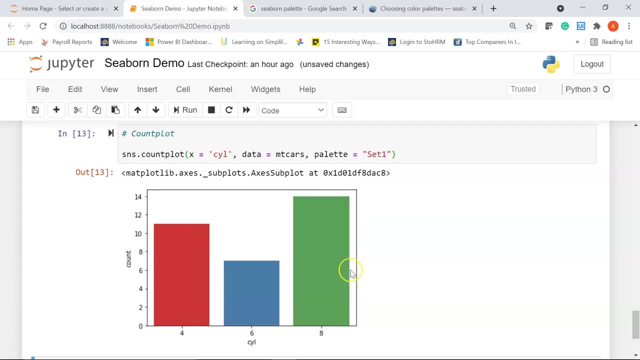 the x-axis and on the y-axis. you have the count. you can see here there are more number of vehicles that have eight cylinders and there are less number of vehicles or cars that have six cylinders, and actually you can count it as well. so you can see, here there are. 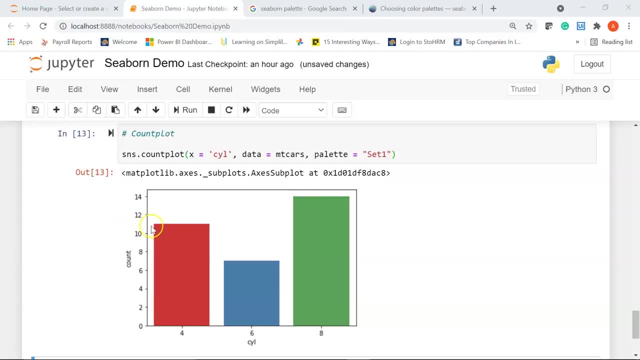 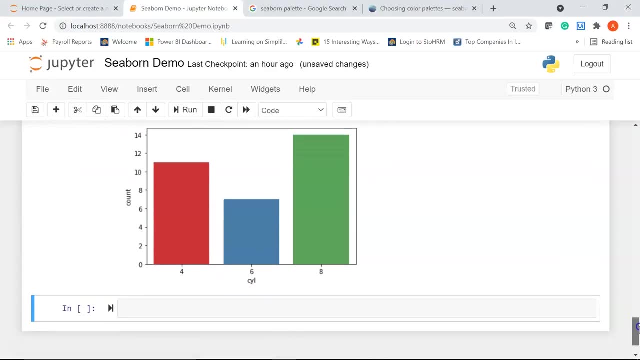 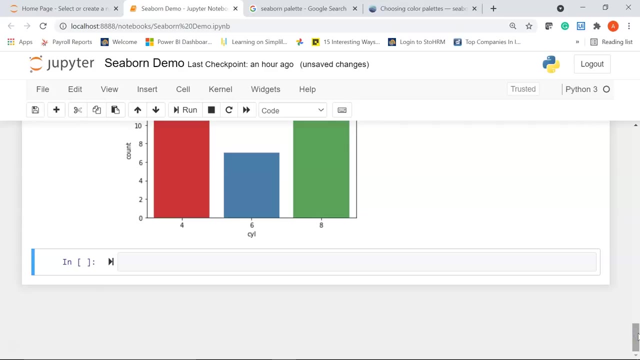 14 cars that have 8 cylinders, there are 11 cars that have 4 cylinders and there are 7 cars that have 6 cylinders. all right now, moving ahead, the next count plot will show the number of cars for each carburetor. so for that, i'm going to say: 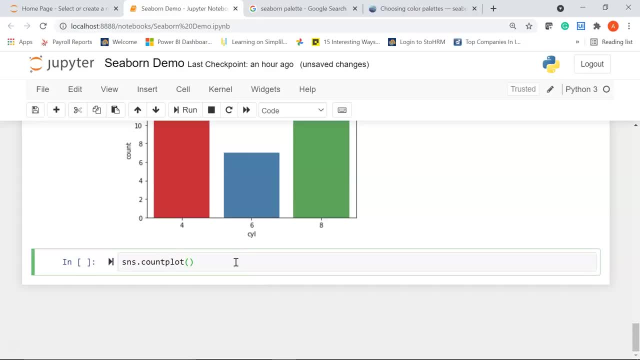 sns dot count plot. my x-axis will now have the variable carburetor. i'll see data equal to empty cars and my palette. i'll set it to set one. let's say set two. now let me run it. you can see it here. on the x-axis we have the different number of carburetors: one, two, three, four, six and eight, and you can see we have more number of cars that have two and four carburetors and there are very few vehicles that have six and eight carburetors here. so let's had four more carburetors and create another. 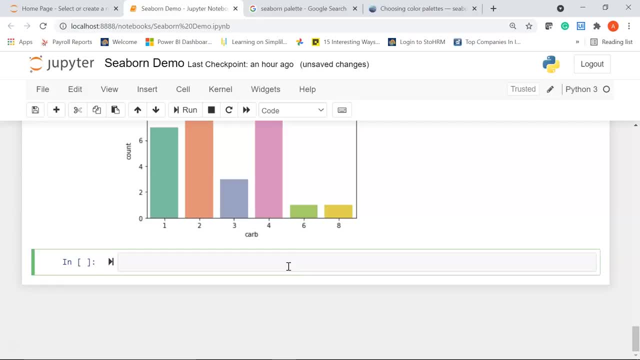 carburetor cool now moving ahead. so the python cbon library allows you to create horizontal count plots where the feature column is on the y-axis and the count is on the x-axis. let me show you how to create a horizontal count plot. i'll say sns dot count plot. 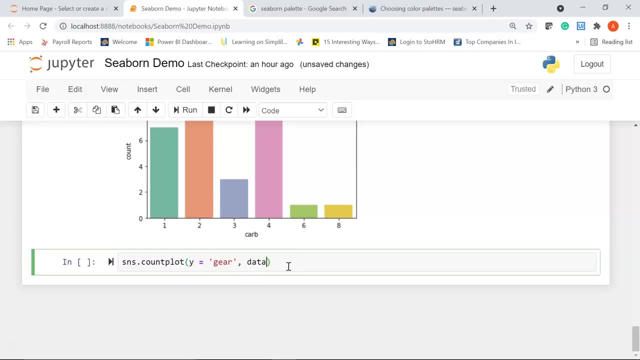 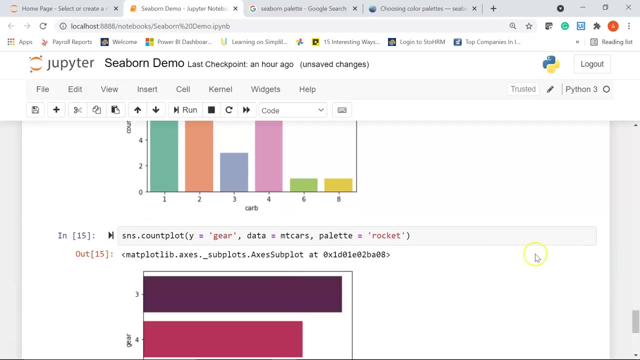 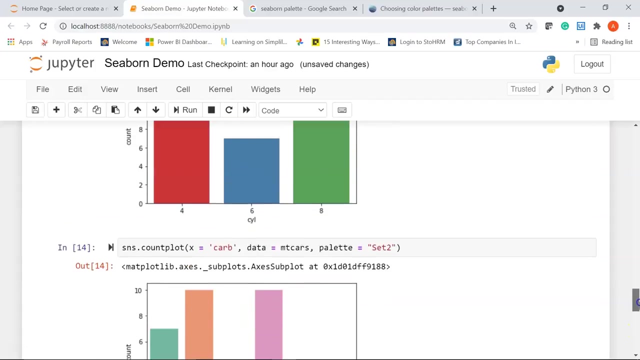 gear, i'll say data equal to empty cars and set my palette to, let's say, rocket. let me run it. okay, you see here this is a horizontal count plot. if you compare it with the above one, these were all vertical count plot as in the bars were vertically aligned. 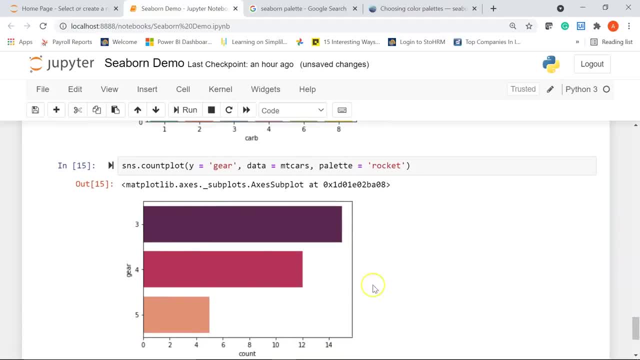 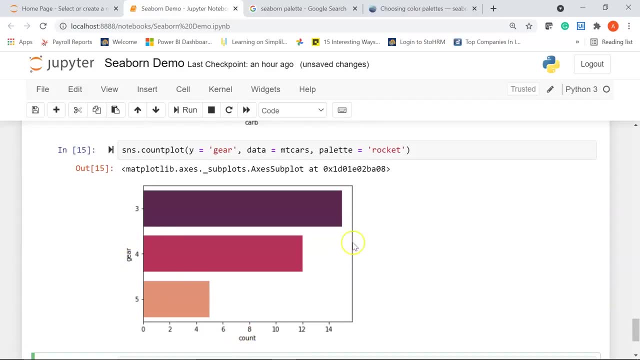 but here you can see the bars are all horizontally aligned and on the y-axis you have the gear column and on the x-axis you have the count. so if you mark here properly, you can see there are 15 vehicles with three gears, there are 12 vehicles that have four gears and there are total five vehicles with. 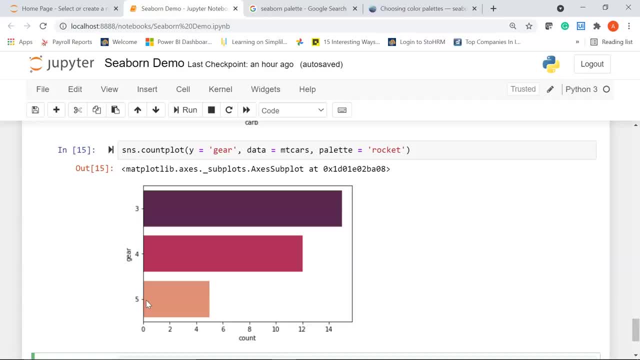 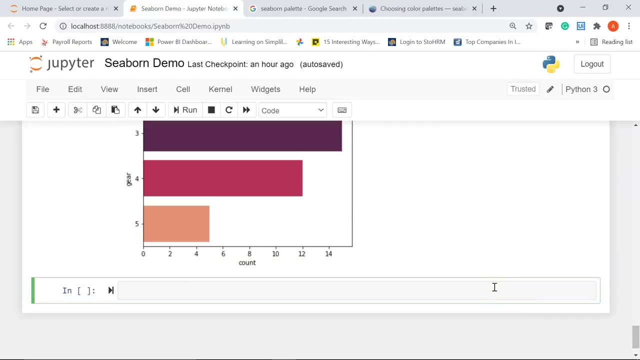 five gear. now you can also create a grouped count plot using the hue parameter. so the hue parameter accepts the column name for color encoding. now let's build a count plot that shows the number of cars for each category of gears grouped by the number of cylinders. so we are going to group. 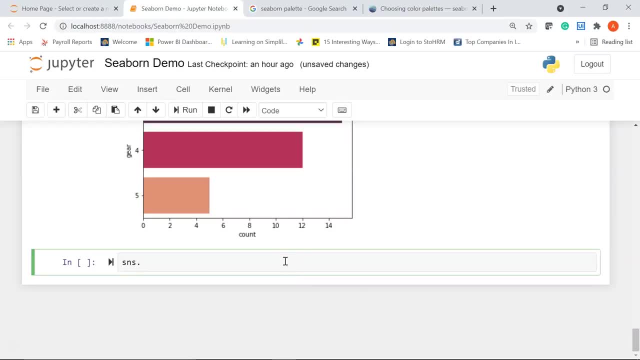 based on the number of cylinders. let me show you how to use the hue parameter. for that i'll say sns, dot and count plot. in the x-axis i'll have my gear column. then i am going to pass my hue parameter that will have the cylinder column, or the number of cylinders for each vehicle. 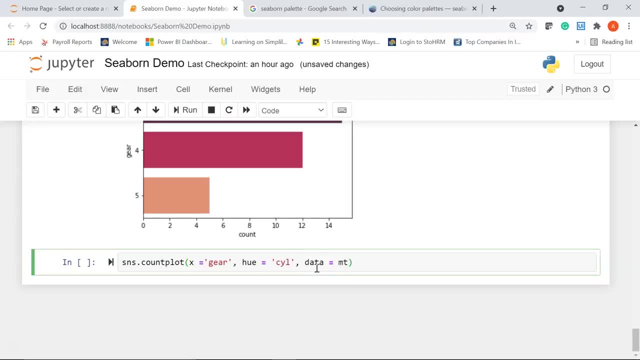 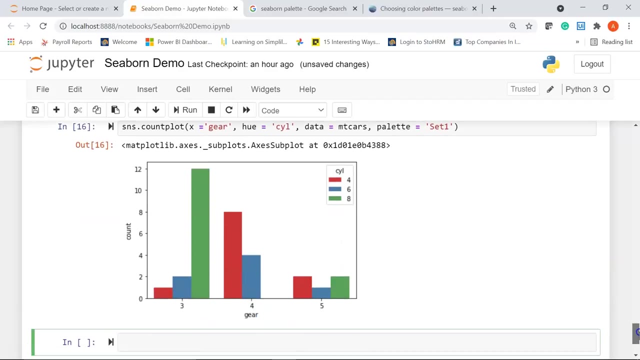 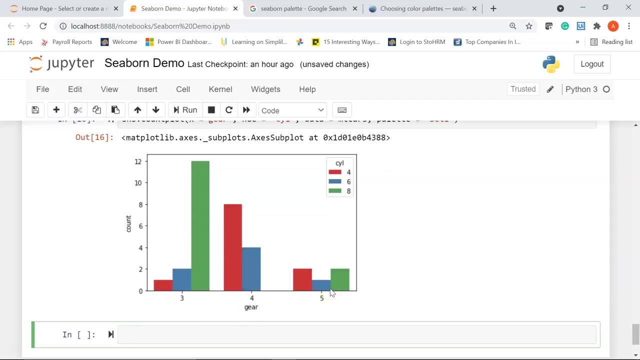 i'll pass my data frame using the data argument as empty cars and say palette. i'll set my palette to set one. let's run it. if i scroll down you see here we have a count plot. on the x-axis you have three, four and five gears of the different vehicles and for each gear you have the bars. 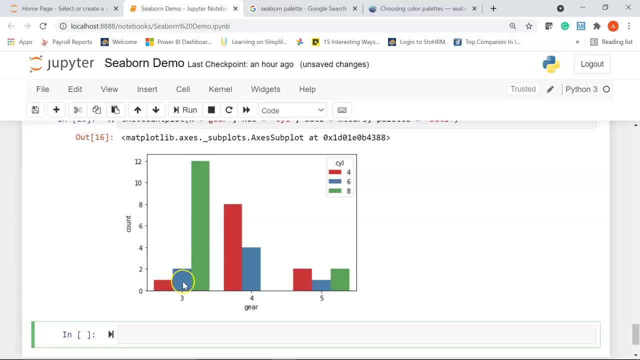 that represent the number of cylinders. so, for vehicles that have three gears, we have majority of the vehicles having eight cylinders. similarly, for vehicles that have four gears, we have most of the vehicles with four cylinders and, if you compare, for the cars that have five gears, so we have equal number of vehicles that have four and eight. 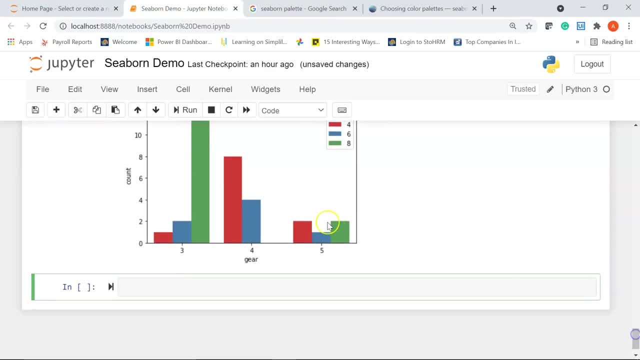 cylinders and then we have one vehicle that has six cylinders. cool, now moving ahead. so the seaborn library supports the distpl Лю Seaborn Re baker component, as you can see, because it comes with a distplot function that creates the distribution of any continuous data. 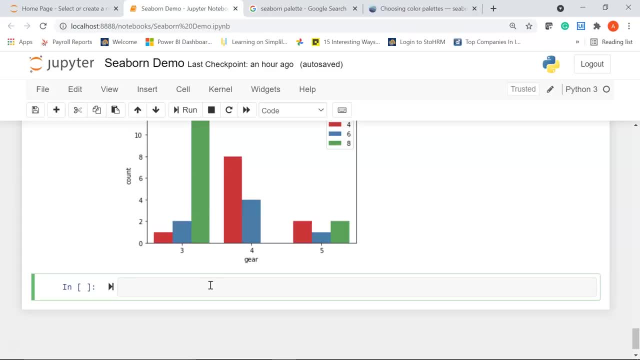 let's create the distribution of miles per gallon of the different vehicles or the cars. the mpg matrix measures the total distance the car can travel per gallon of fuel. so here I'll give a comment. as distplot, which stands for distribution plot, I'll say snsdistplot. 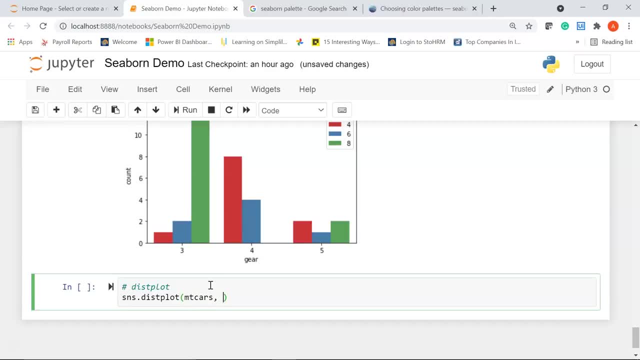 I'll pass in my data frame name, that is empty cars, give a period and say mpg, which is my column name. then I'm going to define the number of bins that I want- let's say 10- and then I'll use the color argument and I'll say, let's say g, which is for green. 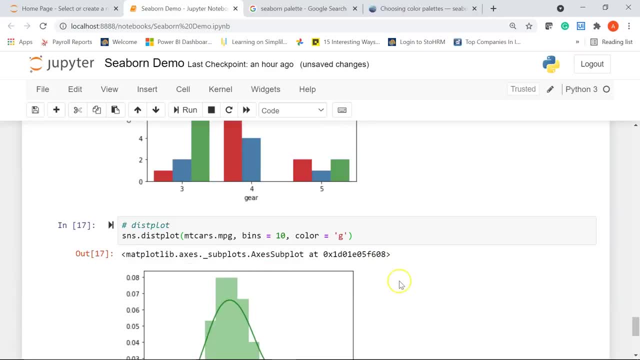 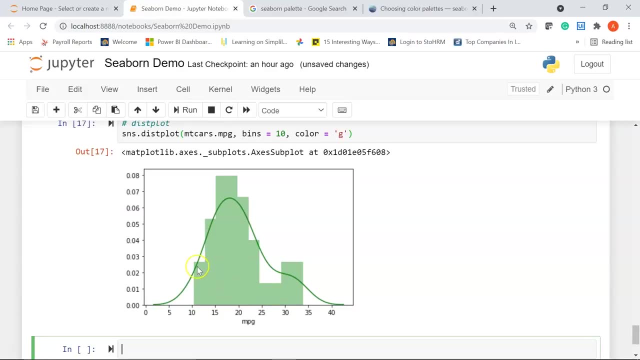 and let's run it now. there you go. if I scroll down, you can see we have a nice distribution plot. so these are all histograms and you can see we have a smoothed curve and this shows the distribution of miles per gallon that is present in our data set. alright, now moving ahead. 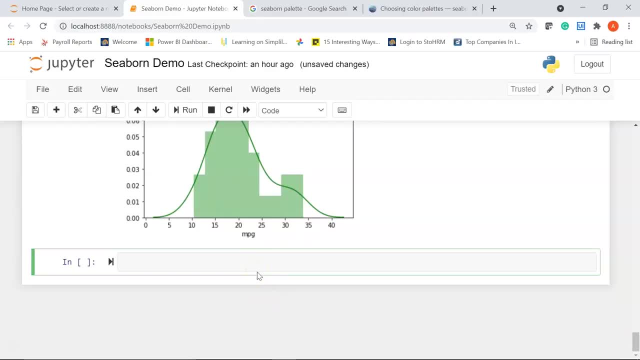 you can also create heat maps using the seaborn library, and so the heat maps will let you visualize matrix like data. the values of the variables are contained in a matrix and are represented as colors. you can create a correlation heat map, which is a graphical representation of a 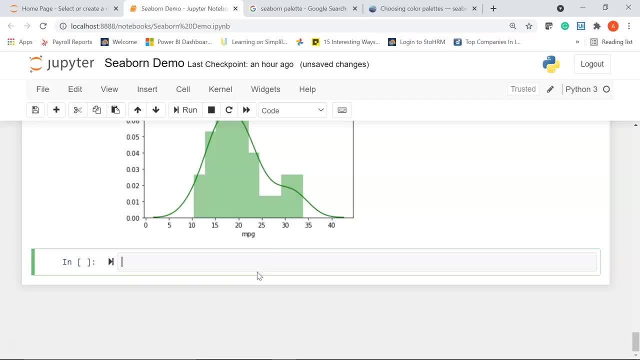 correlation matrix representing the correlation between different variables. so in our example we will create a heat map where you can find the correlation between each variable in the empty cars data set. I'll just give a comment as heat map, I'll say SNS and I'll use the heat map function. 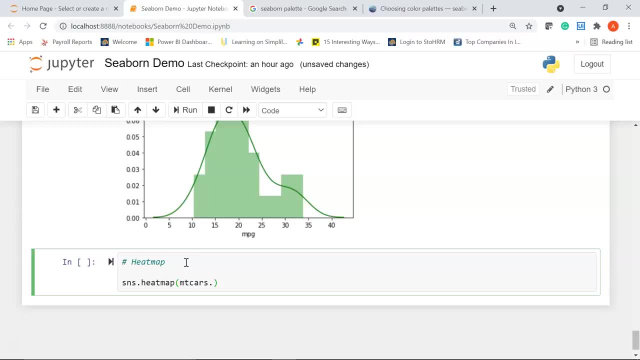 I'll pass in my data frame name that is, empty cars, followed by a function called CORR, which is for correlation. then I'll say: C bar is equal to true, so the C bar argument is used to draw the color bar. then I'll say: line widths. 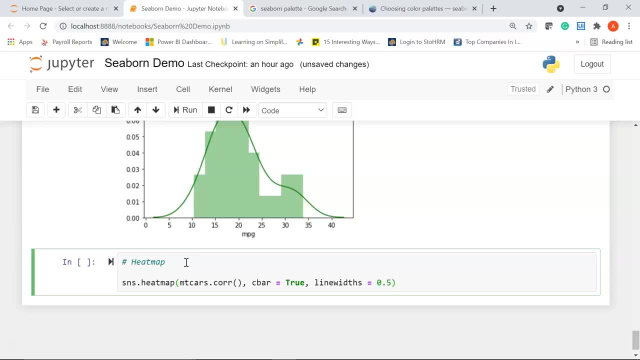 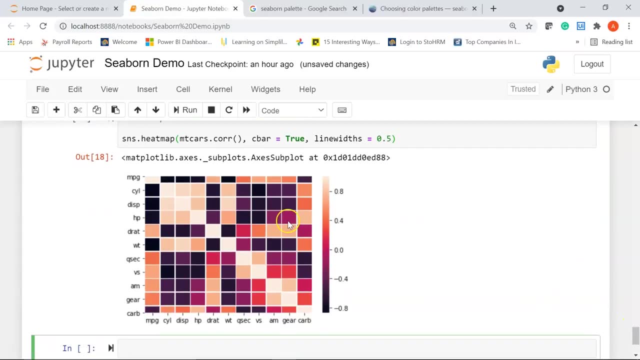 I'll pass it as 0.5. let's run it. there you go. here you can see we have a nice heat map and on the right side you can see the color bar that starts from minus 0.8 and goes up to plus 0.8. 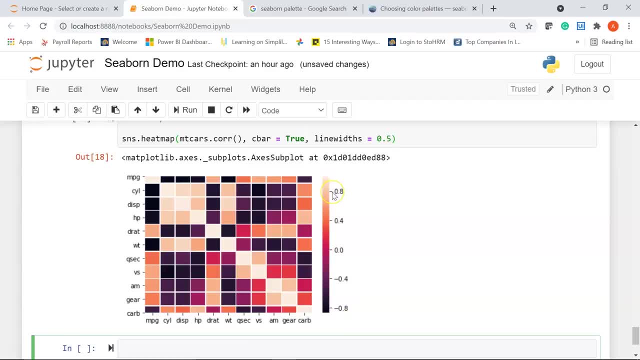 so this ranges between minus 1 and plus 1. and the bars or the cube you can see that have a lighter color, have a positive correlation and the ones that are dark have a negative correlation. so for example, you can see here for cylinder and mpg the color is really dark. 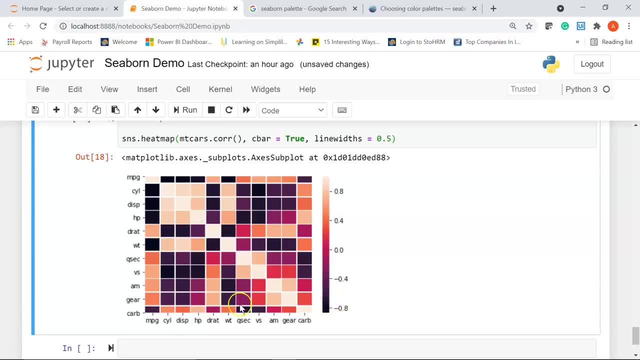 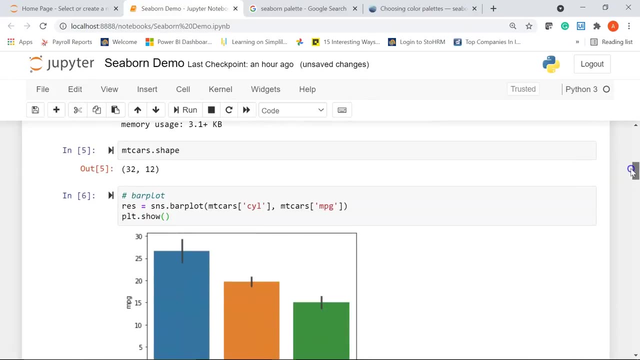 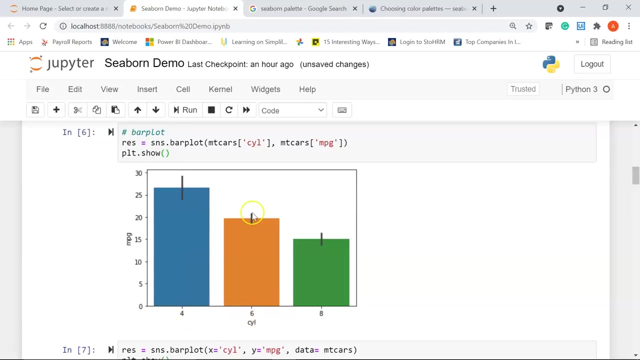 which is around this region minus 0.8. this means when the number of cylinders in the car increases, your miles per gallon decreases. and this we also had seen in our first bar plot. this one you can see here: whenever the number of cylinders increased, your miles per gallon had decreased. 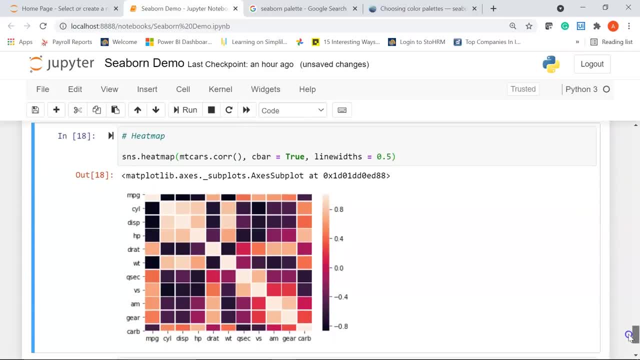 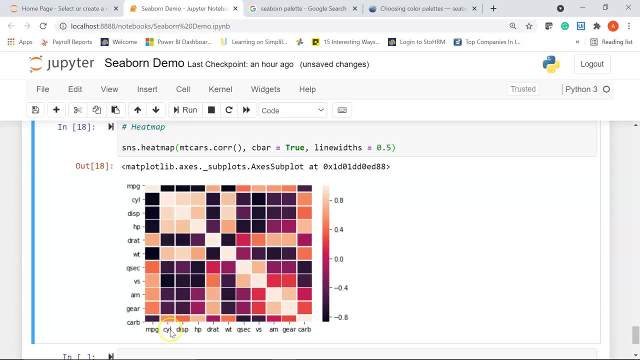 and this is what has been depicted in our correlation map or the heat map. but if you see from here, for cylinder and displacement there is a positive correlation which comes around this color bar range. similarly, there are other features in the data set. for example, if you compare for 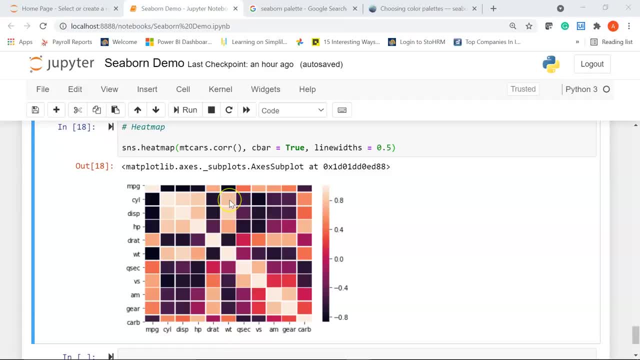 the weight of the vehicle and the number of cylinders. there is a positive correlation which means when the weight of the vehicle increases, the number of cylinders present in the vehicle also increases, and the others? you can also compare and find out the correlation based on this color bar. 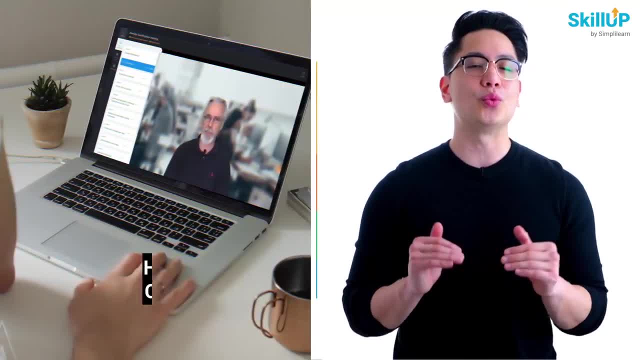 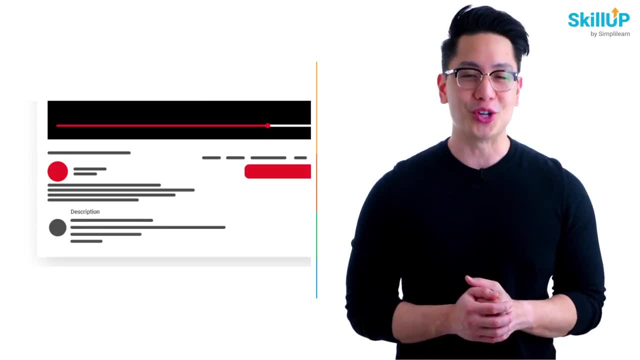 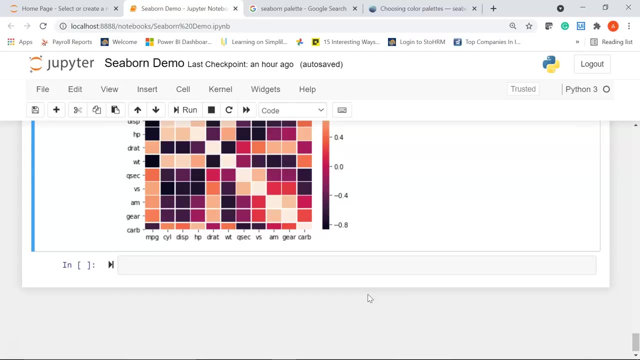 choose from over 300 in demand scales and get access to 1000 plus hours of video content for free. visit scale up by simply learn. click on the link in the description to know more. okay, now let's move ahead. the seaborn scatter plot function helps you create plots that. 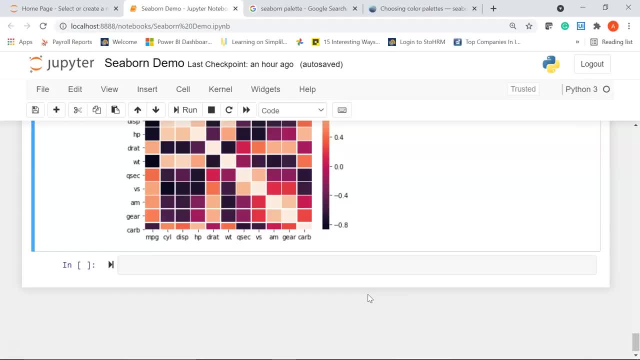 can draw relationships between two continuous variables. so to understand about scatter plots and other plots and plot functions, henceforth we are going to use iris plot data set, so let's go ahead and load the iris plot data set. I will say: iris equal to sns. dot load underscore. 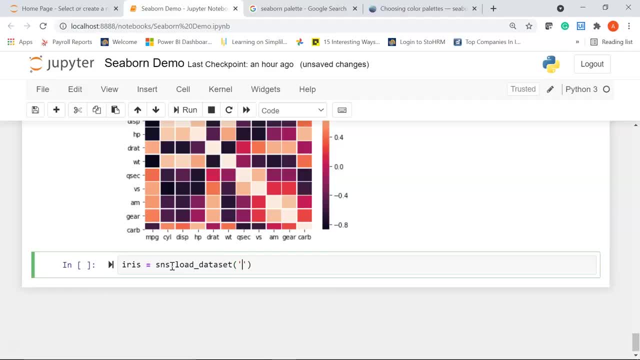 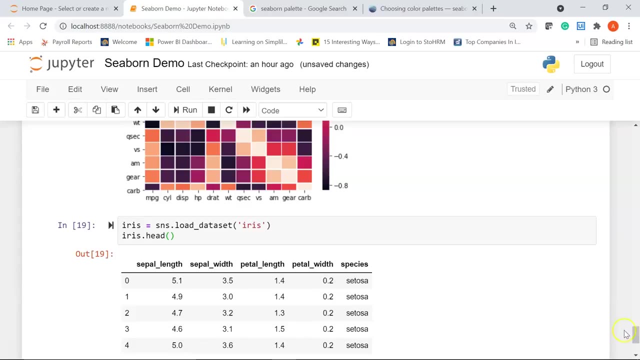 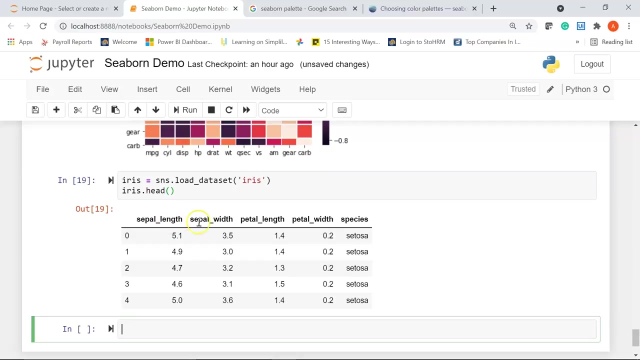 data set. so this iris plot data set is already inbuilt into the sns or the seaborn library. now we will go ahead and print the first five rows from the data set. there you go here. you can see here there are total four feature variables. you have the sepal length. 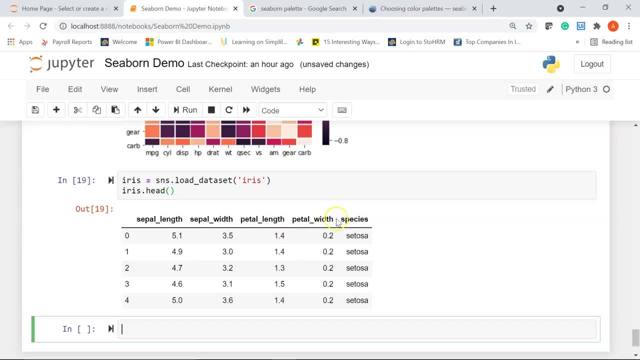 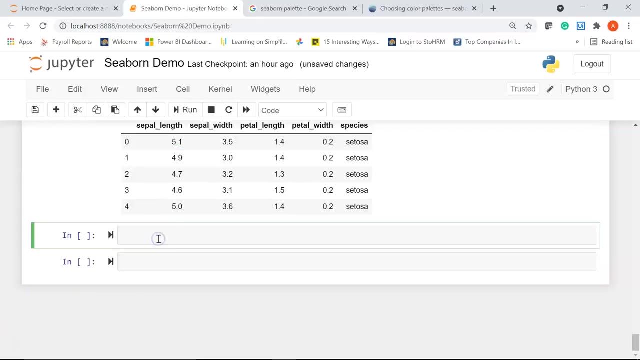 sepal width, petal length and petal width of the three species of flower, that is, setosa virginica and versicolor. so using this data set, we are going to see the rest of the seaborn plotting functions. first let me go ahead and print the different species of flower and the 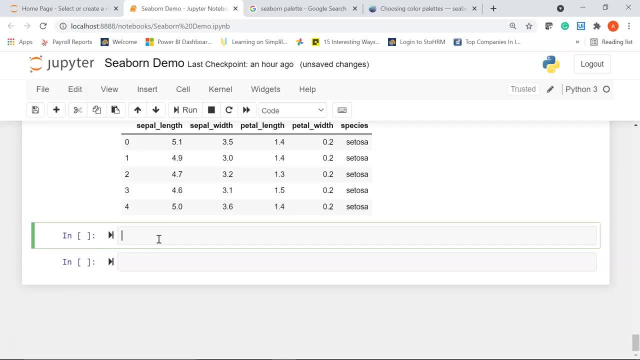 count for each of the species of flowers that we have in our data set. I will say iris, within square brackets. I will pass in the output or the target variable, that is species, and I will use the function that is value underscore counts. let's run it. there you go. so we have. 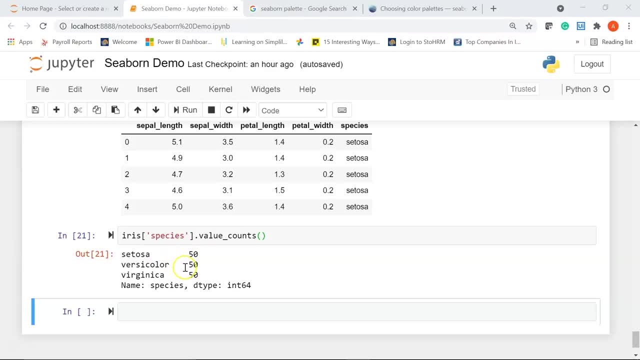 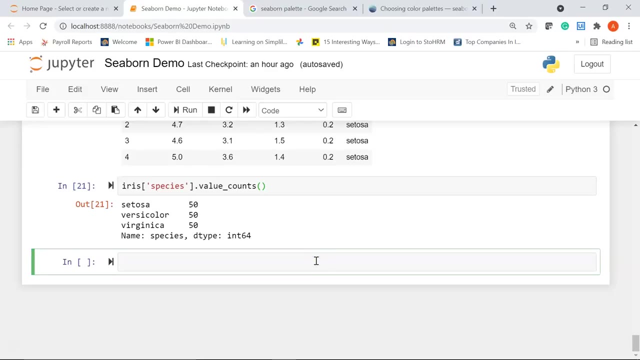 50 flowers of setosa type, again 50 flowers of versicolor species, and then we have another 50 flowers of type virginica. so there are total 150 flowers present in our data set. all right, I will create a scatter plot to show the relationship between sepal length and. 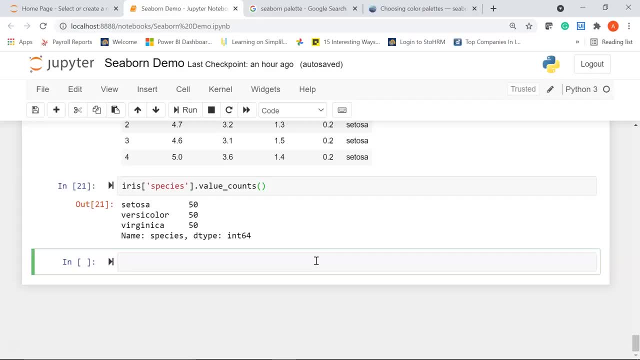 petal length for different species of iris flowers. so I will say sns dot, followed by the scatter plot function. in the x axis I will say sepal length column. give a comma. I will pass in my y axis with petal length, then I will say data. 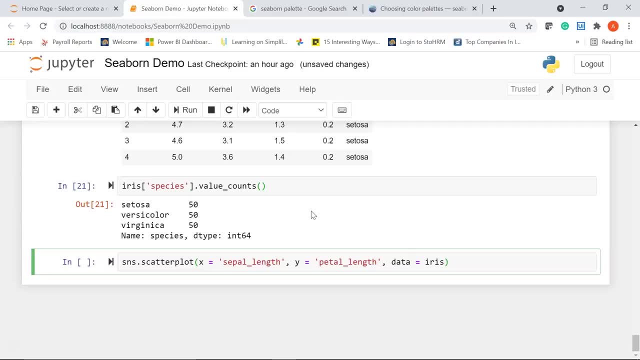 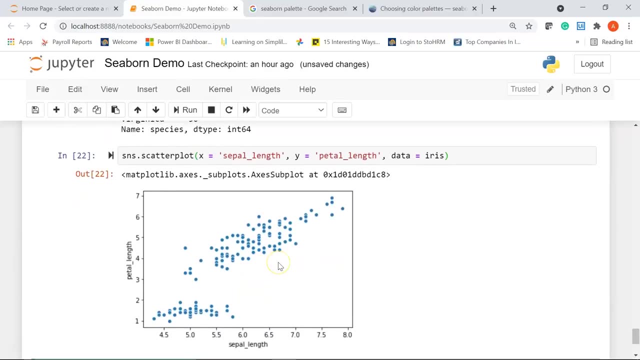 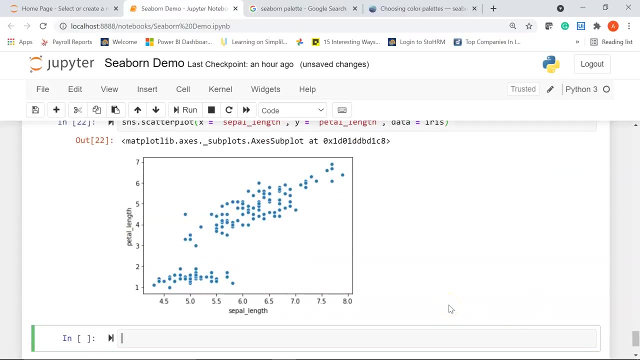 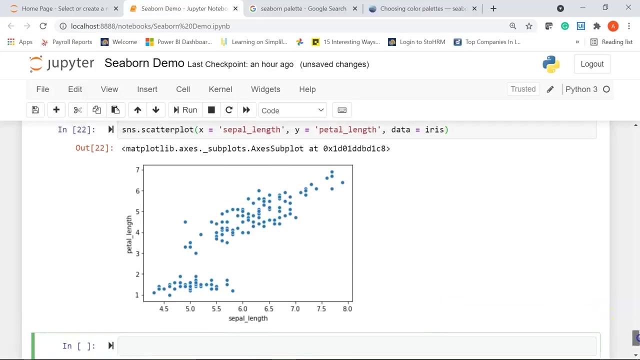 equal to iris. now let's run it. you can see here- this is my scatter plot between sepal length and petal length. now you can classify the different species of flowers using the hue parameter as species in the function. so what I will do is I am going to copy my 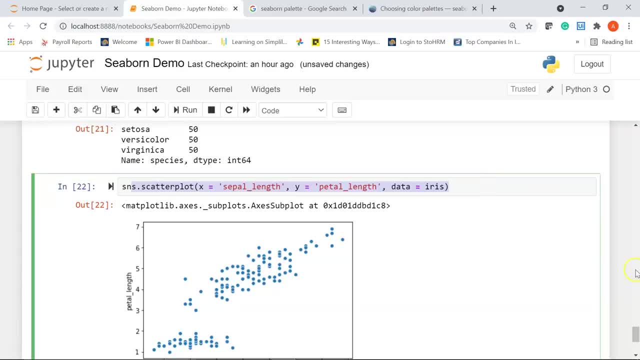 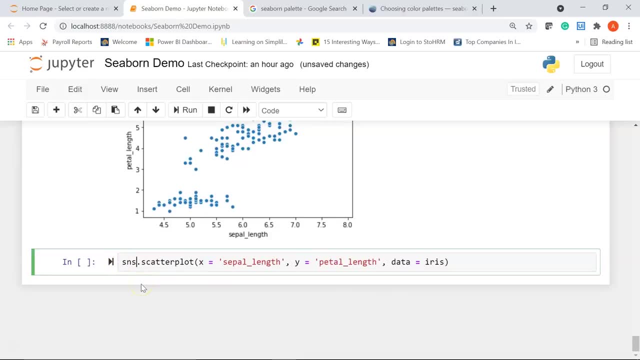 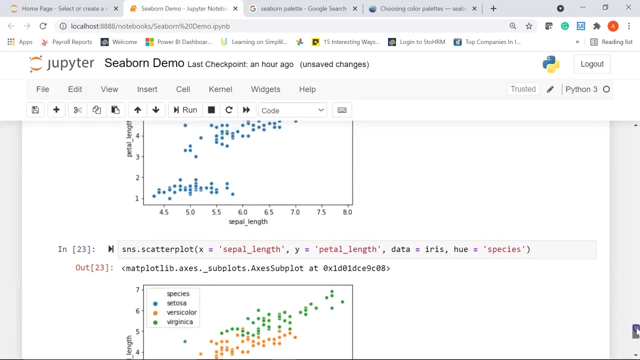 above code. I just paste it here and we are going to edit in this cell itself. I will add a last parameter called hue, and this will have my species column. let's run it and see the difference. there you go. here you can see I have a nice scatter plot. 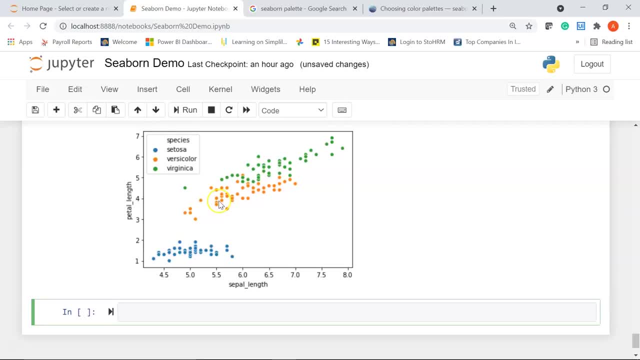 the blue dots are for setosa, the orange dots are for versicolor and for virginica you have the green dots. from this scatter plot you can see that for virginica flowers the sepal length and the petal length are higher than your versicolor, and 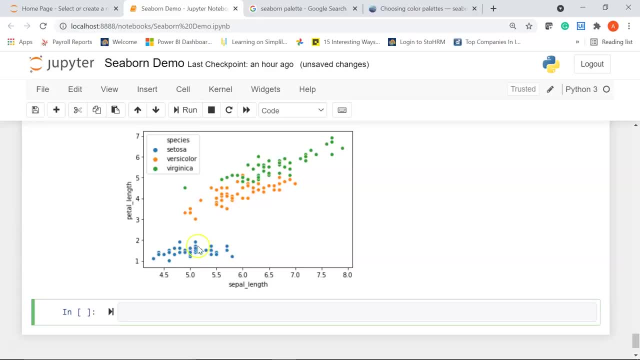 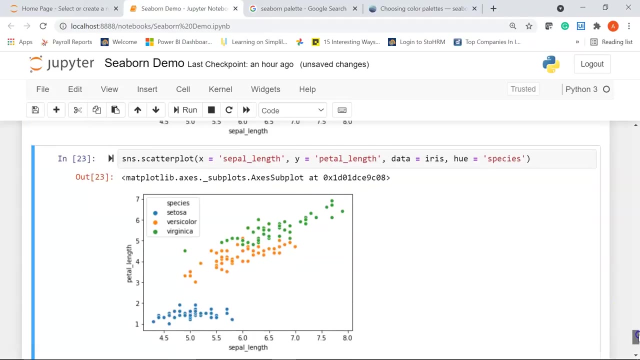 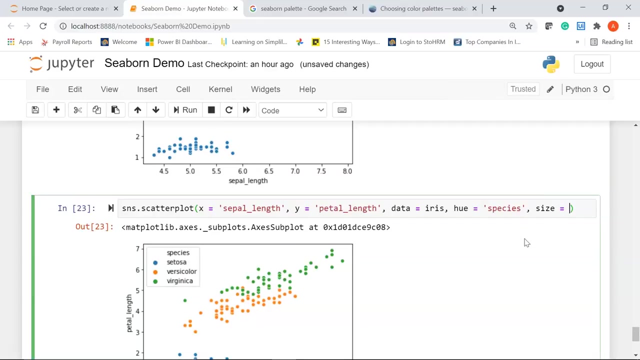 setosa and this region is completely for setosa. so you can see that setosa flowers have lower sepal length and petal length. alright, you can also use another parameter known as the size. that will differentiate the different species of flower in terms of the size of the dots. 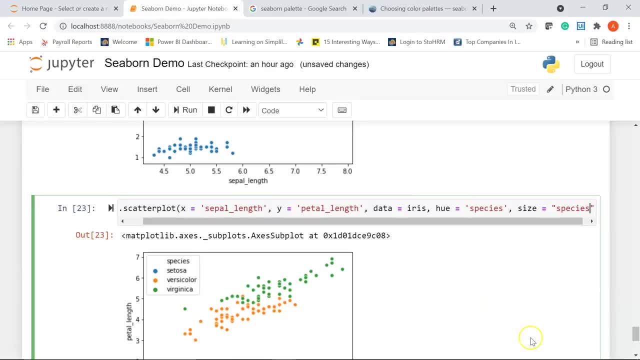 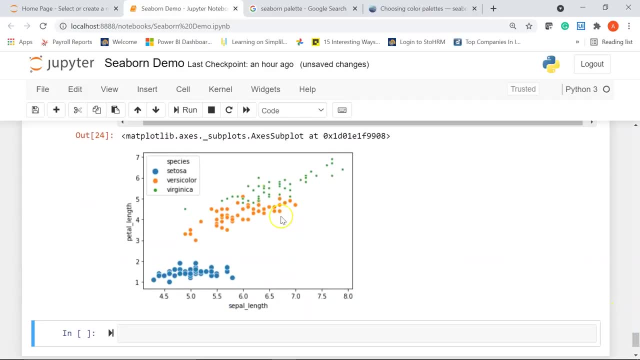 I will say size as species. let's run it. you can see the result. there you go. so here you can see the virginica flowers are in green dots, the size is small, followed by versicolor with medium size dots, and then we have setosa, whose size is. 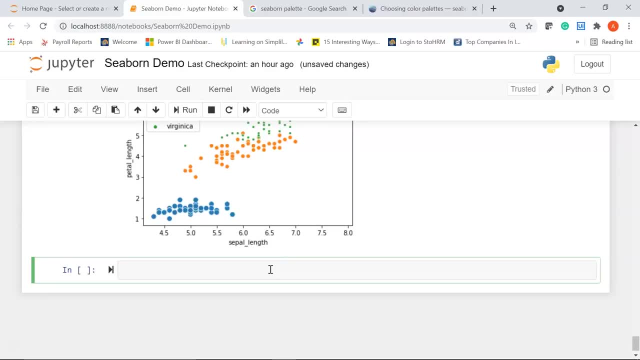 large. now the python seaborn library lets you visualize data using pair plots. that produces a matrix of relationship between each variable in the data set. so let me show you how to create a pair plot. I will say sns dot- pair plot, which is the function. then I will pass in my data frame. 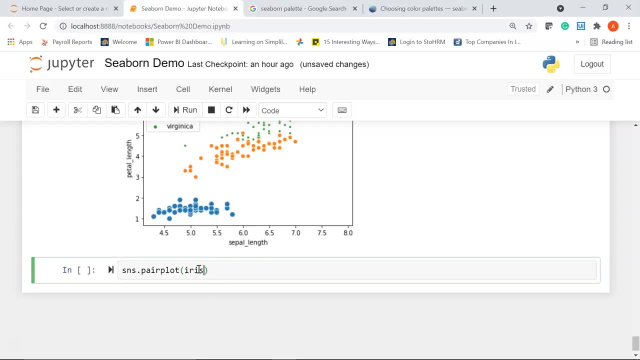 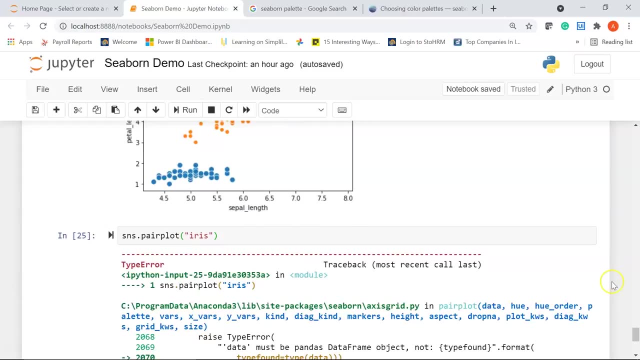 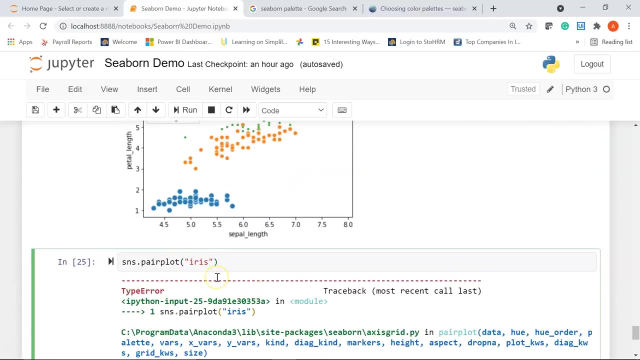 name, that is iris. I will put this iris data frame within double quotes and will run it. ok, there is some error here. lets debug the error. data must be panned as data frame. ok, what I will do is I will just remove the double quotes and will run it. 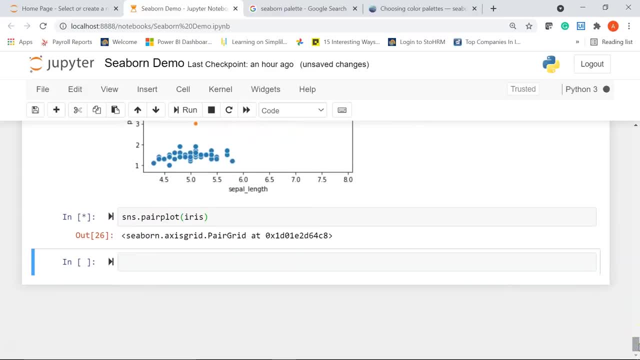 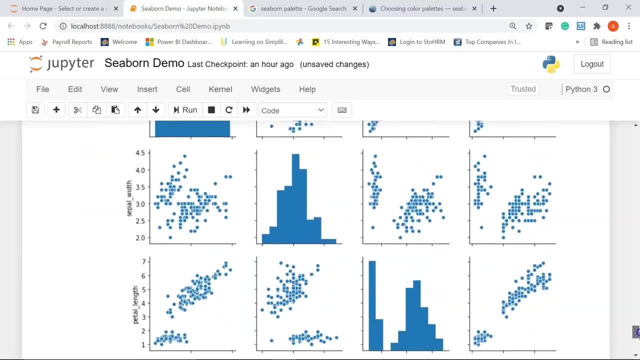 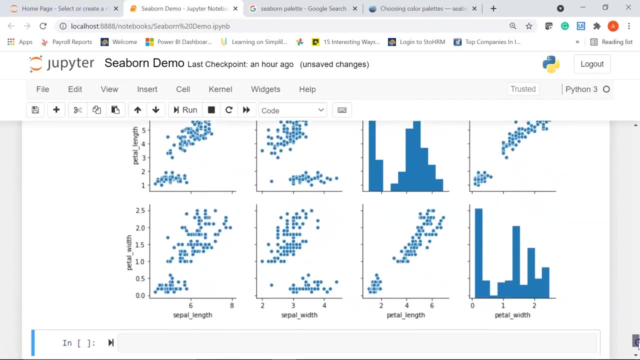 this might take some time to create the pair plot, so just wait for a while. there you go. here you can see we have a nice pair plot. on the y axis you have the sepal length, sepal width, petal length and petal width. similarly on the x axis also. 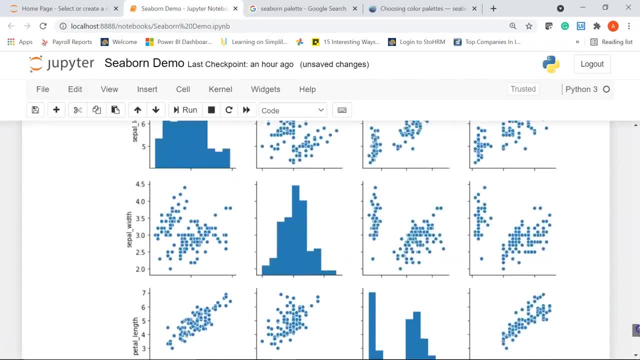 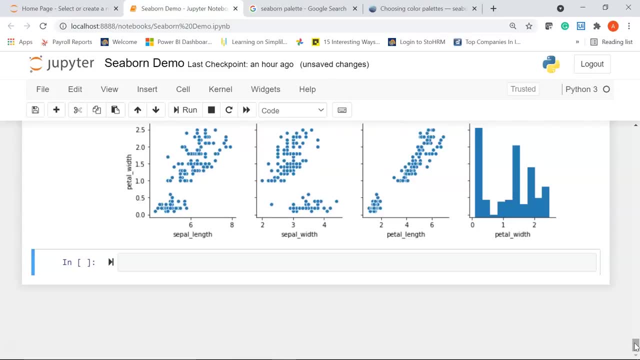 you have the same feature columns. all the diagonal plots are histograms and the rest of the plots are scatter plots. now you can convert the diagonal visuals to kde or kernel density estimation plots and the rest of the scatter plots using the hue parameter. this makes the pair. 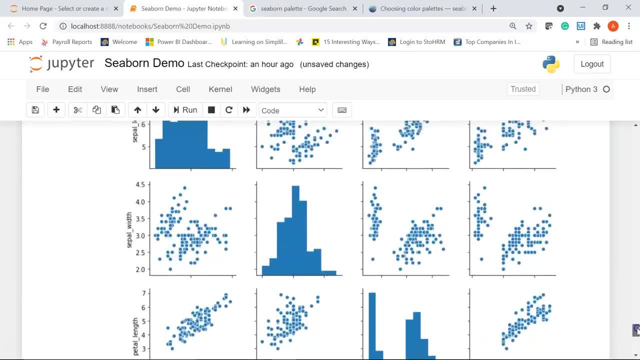 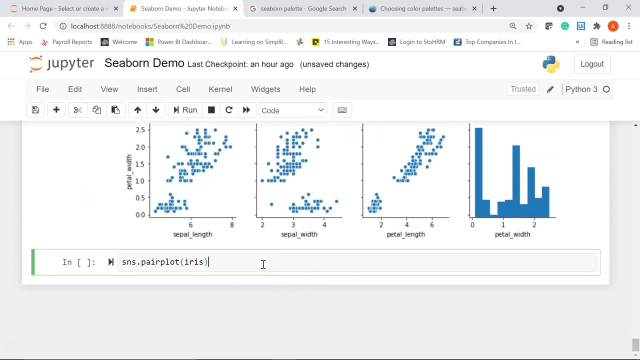 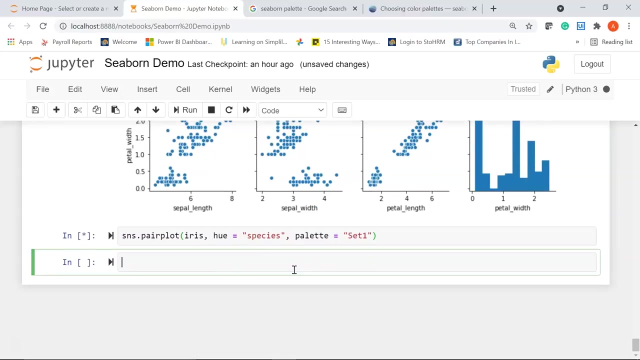 plot easier to classify each type of flower. so I will just copy this cell of code, paste it here and I will say hue equal to species. then I will say palette equal to set1. let's run it and will see the new pair plot. now this might. 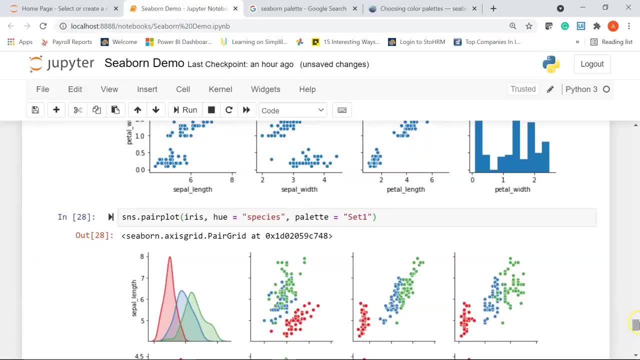 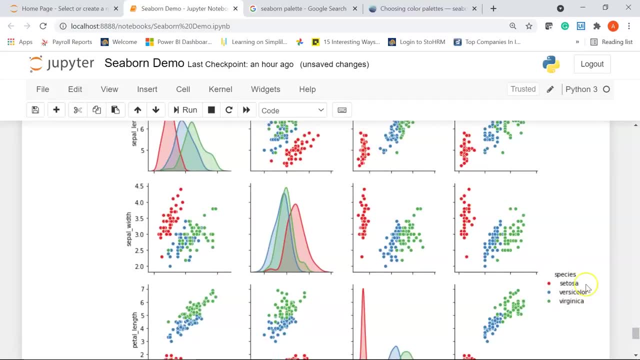 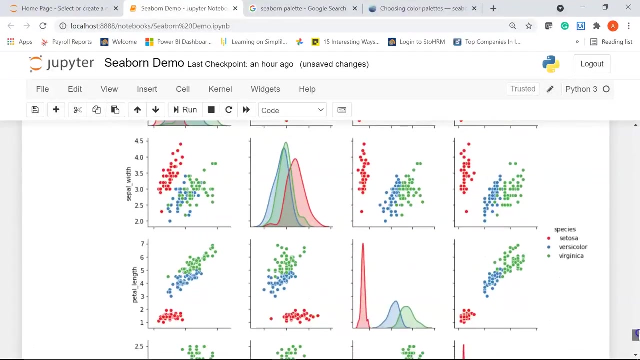 take some time. there you go. so here you have the pair plot ready, and on the right side you can see the different species. the red color dots represent setosa flowers, the blue color dots represent versicolor and the green color dots represent virginica flowers. now, if you 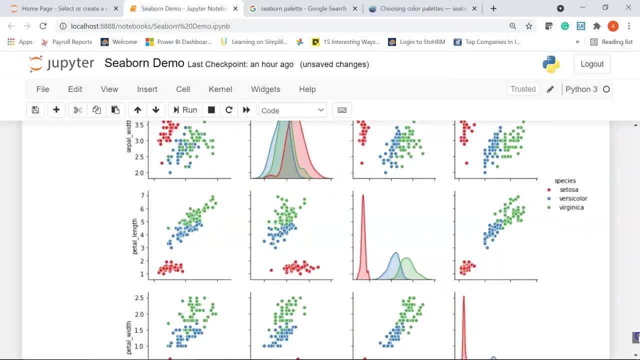 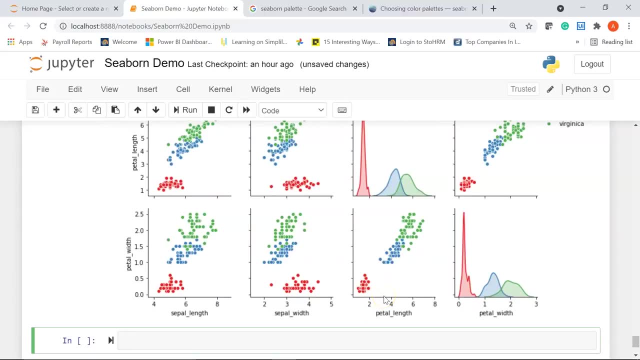 look at this graph, you will find that petal length is the best feature to classify the three different species of flowers with the reason being. you can see here they are very well categorized and they are separated. all the red dots present here in the petal length. 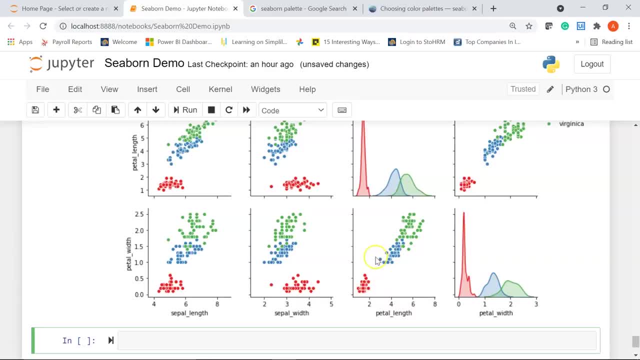 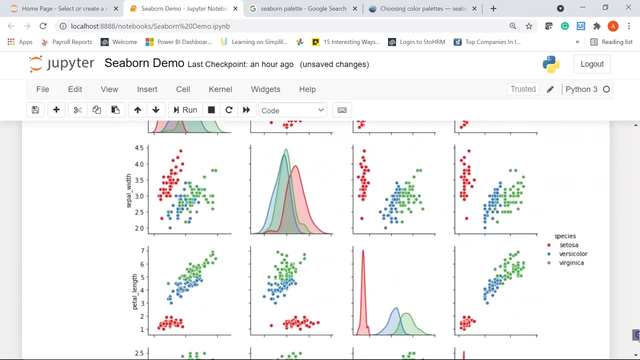 represent setosa flowers around this range. all the blue dots represent versicolor flowers and the green dots are all virginica flowers. so out of the four features- petal width, petal length, sepal width and sepal length- you can take petal length as the 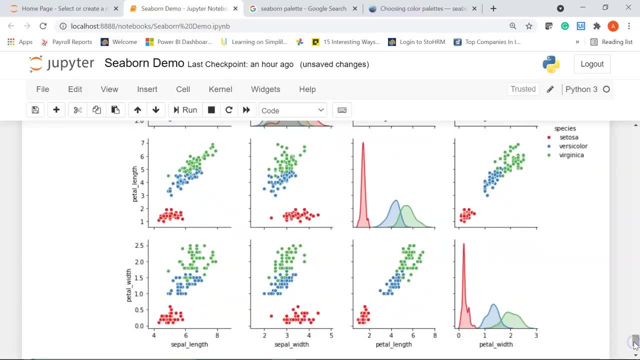 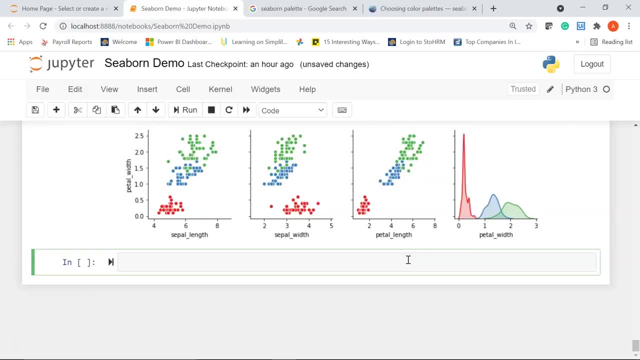 best feature to differentiate between the three species of flowers. alright, now coming to lm plot function. so the lm plot function in the seaborn library draws a linear relationship as determined through regression for continuous variables. so let's create the plot to show the relationship between petal length. 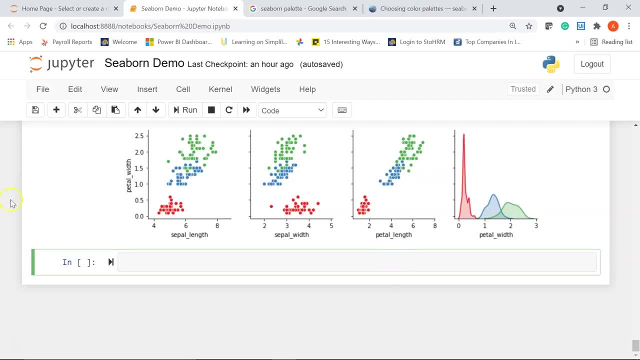 and petal width of the different species of iris flowers. i will just give a comment here. as lm plot i will say sns dot. lm plot in the x axis will have petal length. give a comma. in the y axis i will pass in petal width. 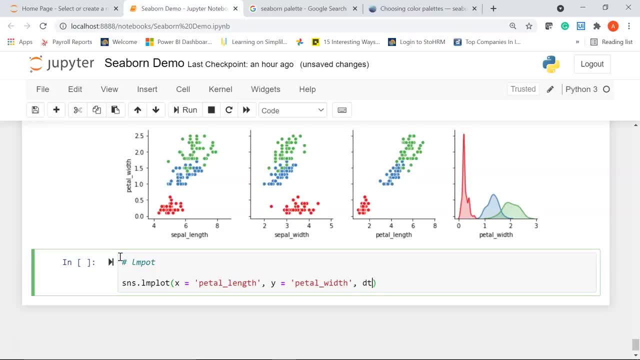 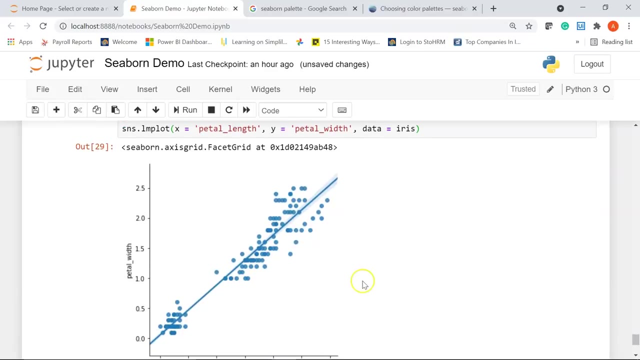 and i will pass in my data frame using the data argument or parameter, which is iris. let's run it. you can see it here. we have a nice plot. the line you see here is a linear regression line. now in this lm plot, you can use the hue parameter to differentiate. 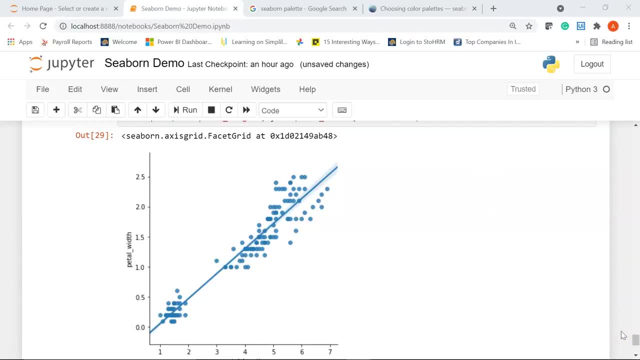 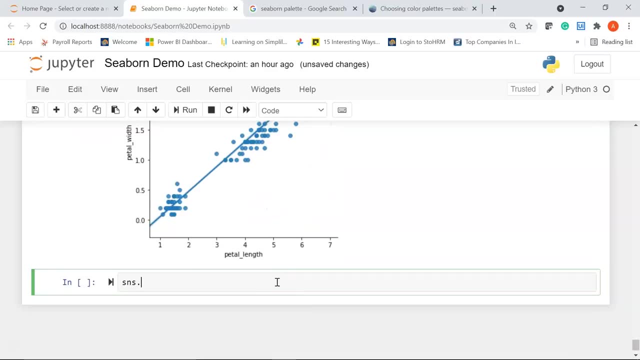 between each species of flowers. you can set markers for different species. let me show you how to do it. i will say sns, dot, lm plot. we will say x as our petal length, give a comma. i will write y as petal width. then i am going to pass the hue parameter. 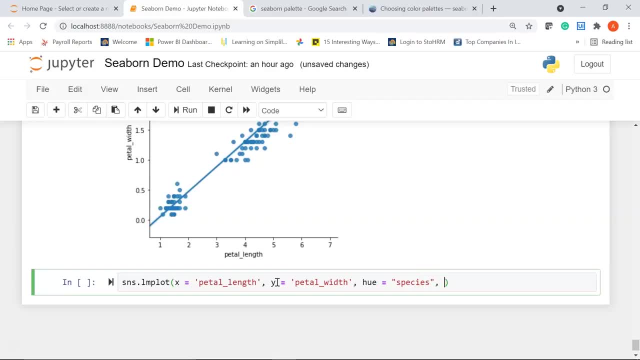 in hue. i will say my column as species, then i will give data equal to my dataset name, that is iris. and now you can pass in markers argument to differentiate the different types of flowers. let's say i want to represent setosa with dot or o. then my next. 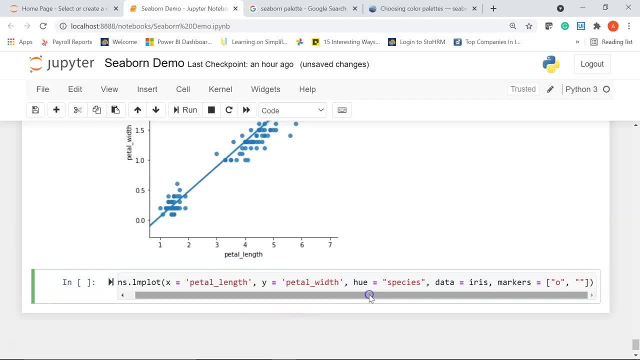 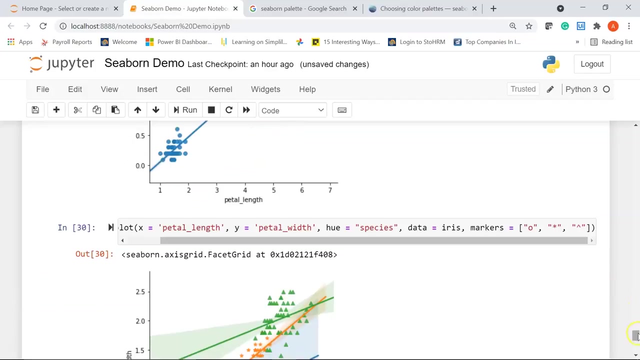 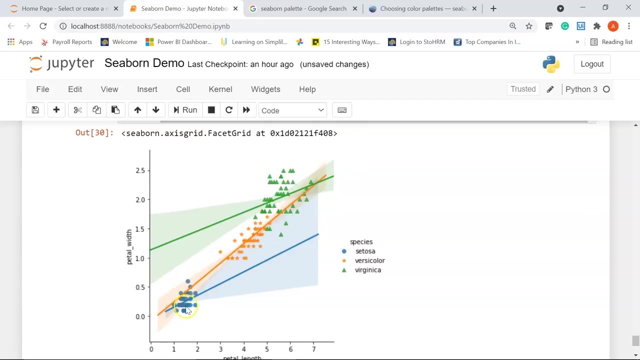 species which is versicolor should be represented with a star symbol and the final virginica species of flowers should be represented with, let's say, this arrow mark. now let me go ahead and run it. there you go. you have three different linear regression lines and the circle. 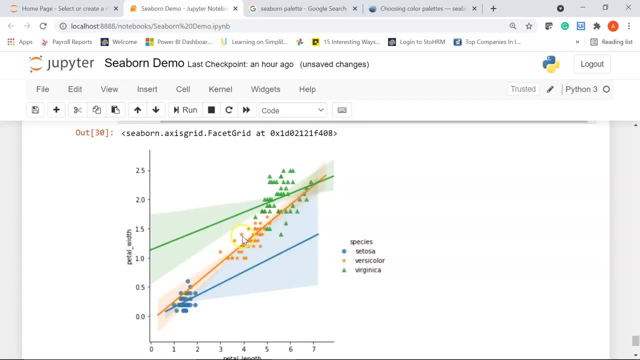 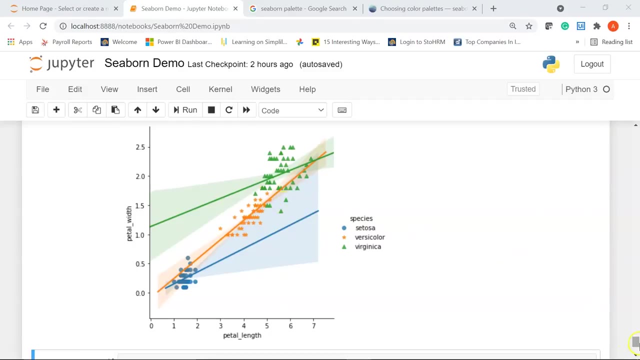 dots in blue color represent setosa, the orange color stars represent versicolor flowers and the triangles represent virginica flowers. so this is how you create a linear relationship between the different types of flowers using the regression line. alright, now let's take a look at the final. 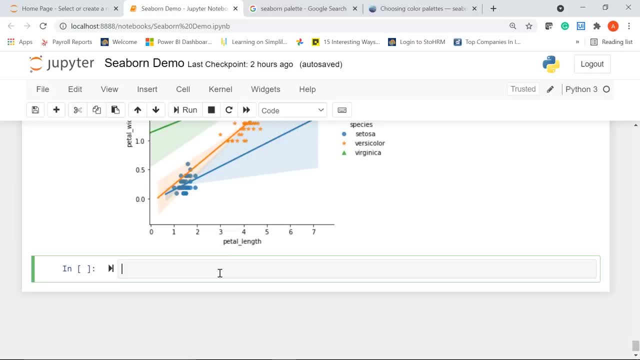 plotting function where we will create a box plot. a box plot, also known as a box and whisker plot, depicts the distribution of quantitative data. the box represents the quartiles of the dataset, the whiskers so the rest of the distribution, except for the outliers. now let's see the distribution of the three species. 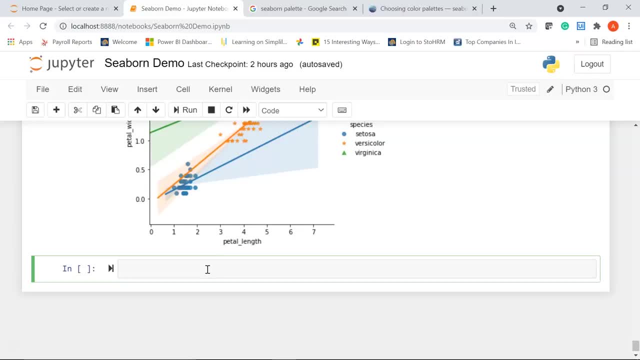 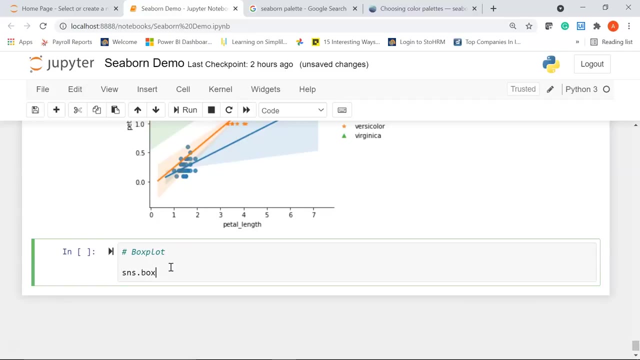 of flowers based on their sepal width. just give a comment: as box plot is the final plot that we are going to see in our seaborn demo, i will say sns dot box plot. in the x axis we will have the species column. in the y axis we will have 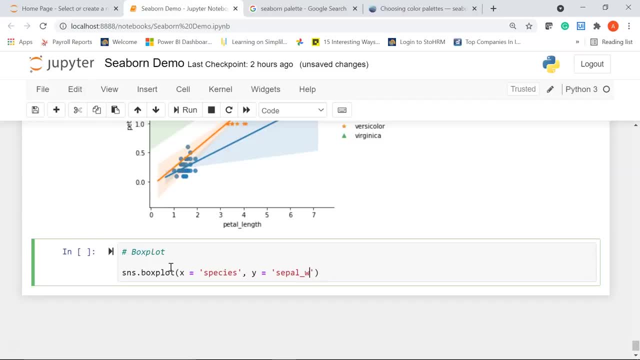 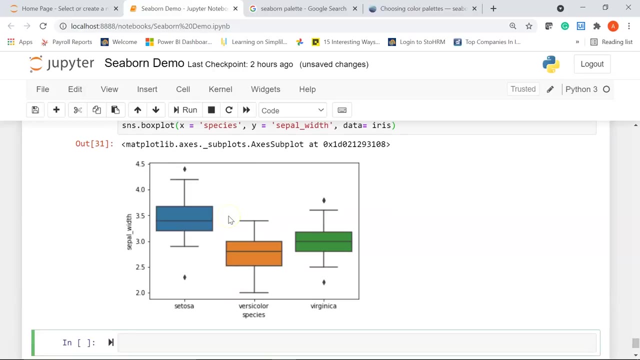 sepal width, then i will pass my data as iris. let's run it. there you go. we have this box plot created at the bottom in the x axis. you can see we have the box plot for setosa flowers, orange for versicolor flowers and green for virginica. 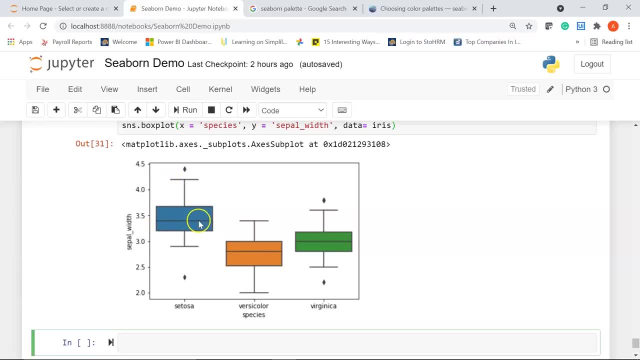 flowers. now this line represents median, which is inside the box, so this is also the median for versicolor flowers. you can compare the median sepal width for each of the flowers from the y axis. this line represents the maximum sepal width value for setosa flower. 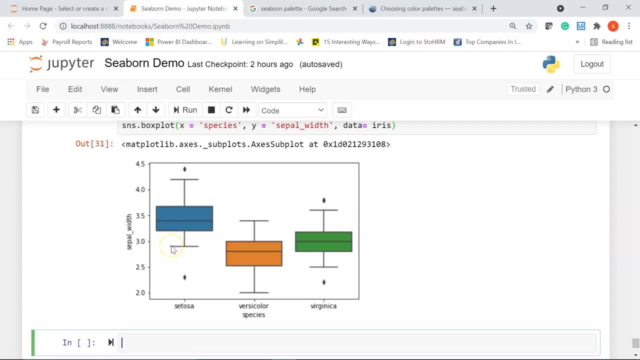 and this line at the bottom represents the minimum length of the sepal width for setosa flowers. now, these dots that you see outside the box plot are called as outliers. the extended lines that are outside the box plot are known as whiskers. alright, so that brings us to the end of this.